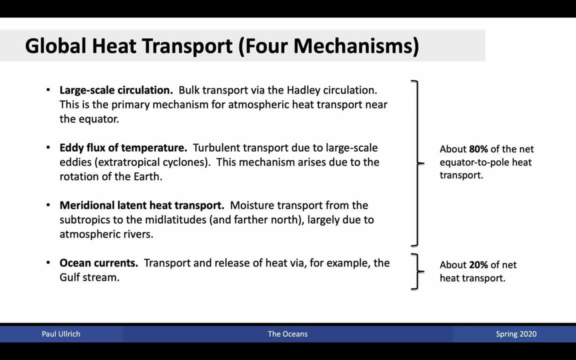 through the large-scale circulation is via dry transport In the mid-latitudes. we also have eddy flux of temperature via sensible heat transport, as well as eddy flux of latent heat via features such as atmospheric rivers. Altogether, these three features of the climate system account for about 80% of the net equator to pole heat transport. 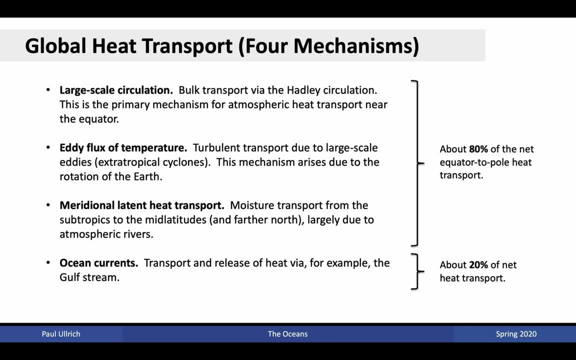 We're now going to focus on the oceans and discuss the remaining 20% of net heat transport. However, this is nonetheless a very important aspect of heat transport, and one which occurs over a very long time. So let's get started. How are the atmospheres different from one another? 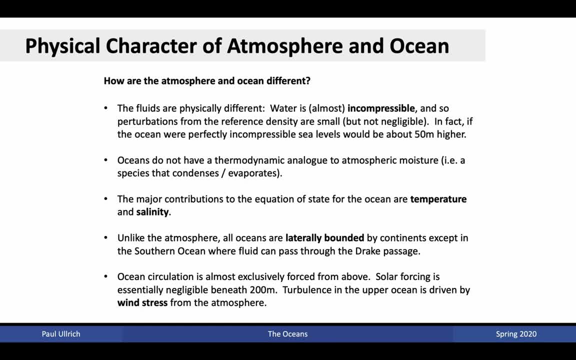 Many of you have not had previous experience with oceanography, so we're going to investigate it in light of what we've learned so far in terms of the atmosphere. Well, how are the atmosphere and ocean different from one another? First of all, the fluids are physically different. 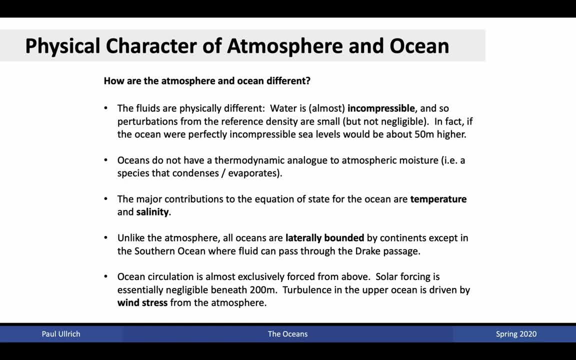 As we know, the atmosphere is made up primarily of a compressible gas. That gas is a mixture of various different constituents, But as a gas it means that it's not a gas. It's a gas that's also compressible As it rises. we have generally that the volume of a particular fluid parcel. 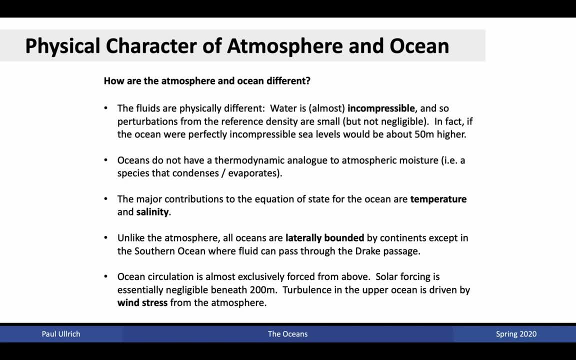 in the atmosphere expands. Water, on the other hand, is almost incompressible, And so perturbations from the reference density- about 1,000 kilograms per meter cubed- are small but not negligible, And we're going to investigate those small differences today. In fact, if the oceans 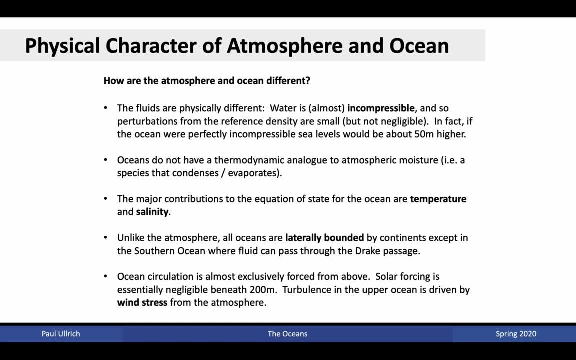 were perfectly incompressible, sea levels would be about 50 meters higher. So obviously we're not going to be able to determine the density of the oceans. We do know that the oceans do not have a thermodynamic analog to atmospheric moisture. You know, in the atmosphere moisture. 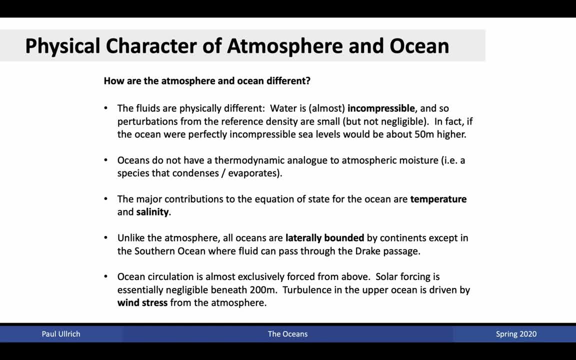 plays an important role because latent heat transport is an important process for moving energy through the system. In particular, moist convection in the atmosphere is responsible for driving instability in the atmosphere, particularly in regions where moisture is high, that is, in the deep tropics. 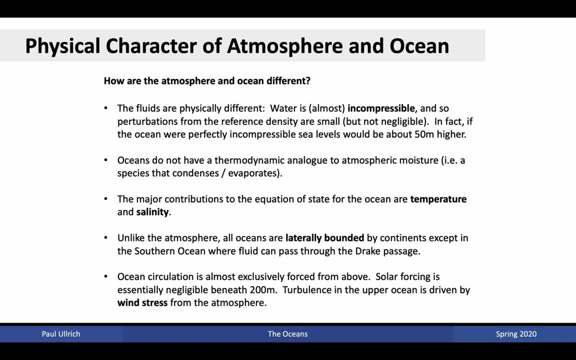 But in the ocean there's no species that condenses or evaporates, In particular not in the same way that moisture does in the atmosphere. In the ocean, the major contributors to the equation of state are temperature and salinity and, to a lesser degree, pressure. But the variations in pressure 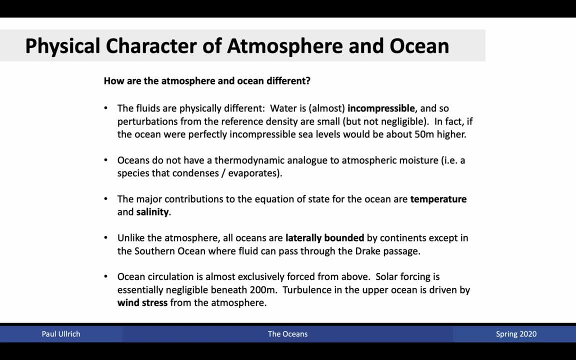 are strongly a function of the depth within the ocean. Horizontally, temperature and salinity are the major contributors that determine the density of ocean water. Unlike in the atmosphere, all the oceans are laterally bound to each other, So we're not going to be able to determine the density of 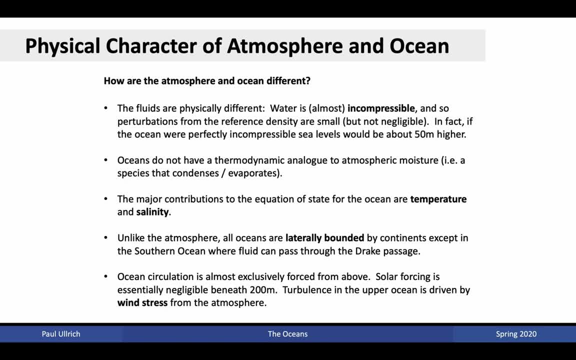 water, in the ocean, In the atmosphere. we can go completely around the Earth and return to our original location, while maintaining ourselves within the atmosphere. Although topography does play a role in driving topographic effects such as mountain lee waves that we've discussed, they do not provide a 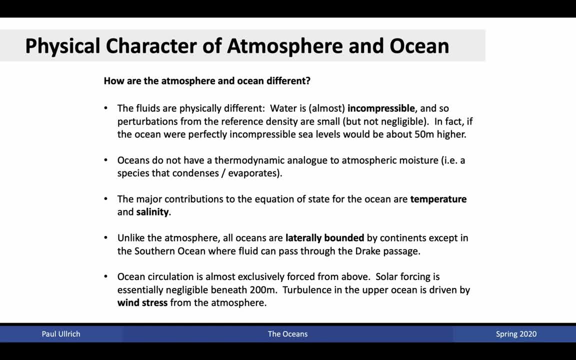 solid barrier by which air cannot pass through. On the other hand, the continents provide lateral bounds to ocean water. That is, the ocean water is effectively bounded as if it was a wall. it cannot proceed through that continental boundary and consequently, you cannot have 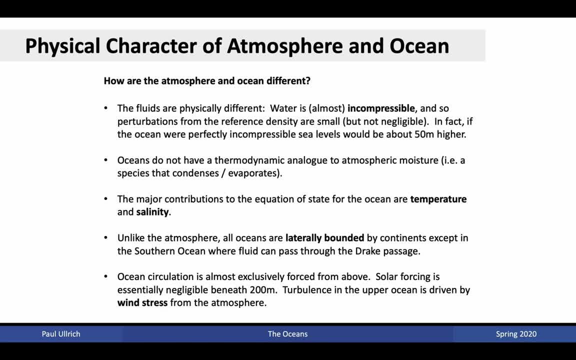 things like jet streams that meander around the whole planet outside of the Antarctic circumpolar current. So it's except in this location in the southern ocean, where fluids are basically laterally bounded and so need to deal with these lateral bounds. The ocean circulation is also almost exclusively forced from above, That is, we have wind-driven forcing. 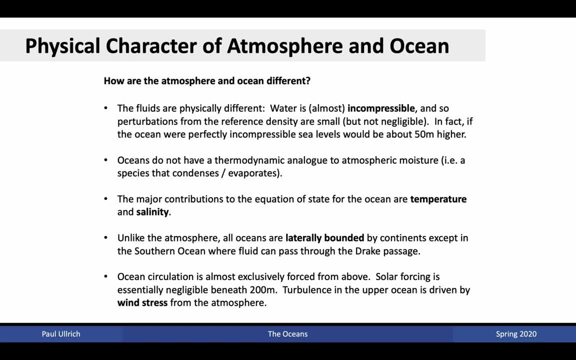 at the top of the ocean layer, which, through frictional effects then, are responsible for driving ocean currents. but heating for the oceans also occurs at the top In the atmosphere. on the other hand, most of the heating actually occurs at the surface, because solar radiation 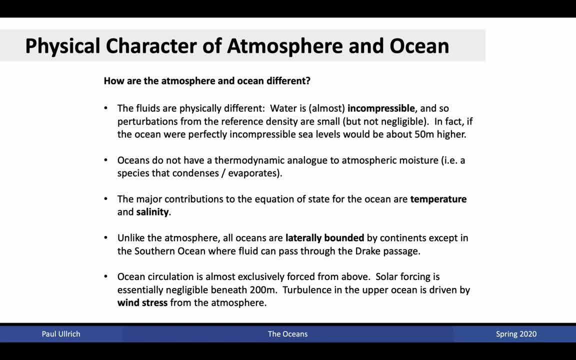 is able to pass through the atmosphere and warm the underlying surface. Consequently, you get significant instability. that occurs because that surface warming is responsible for driving the instability within the atmosphere layer, That is, it makes for warmer temperatures. However, in the ocean, solar forcing is essentially negligible beneath 200 meters With a fluid. 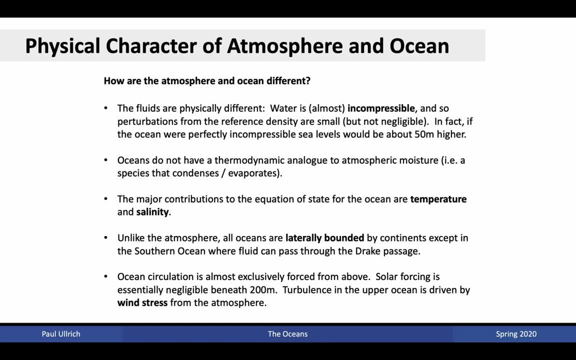 that's heated from above. you don't have heating driving instabilities. In fact, the heating is responsible for driving stability of the ocean. That is, heating of the top of the ocean layer results in a less dense fluid overlaying a more dense fluid, which 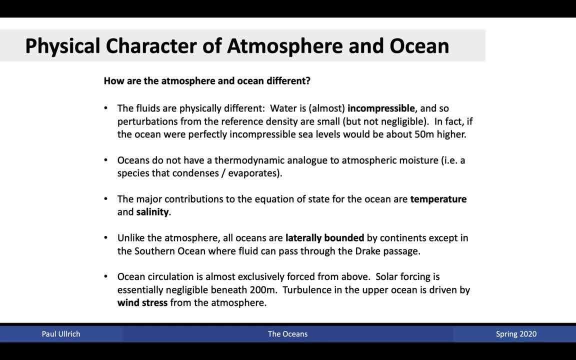 as we're aware from our study of buoyancy, is then responsible for driving stability. However, we have a very turbulent mixed layer at the top of the ocean that is driven by wind stress, and this turbulent layer is also responsible for mixing up the ocean layer. 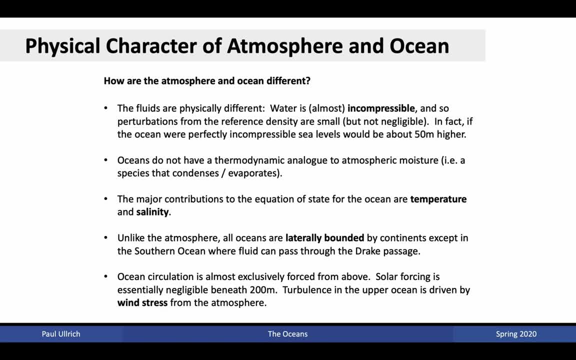 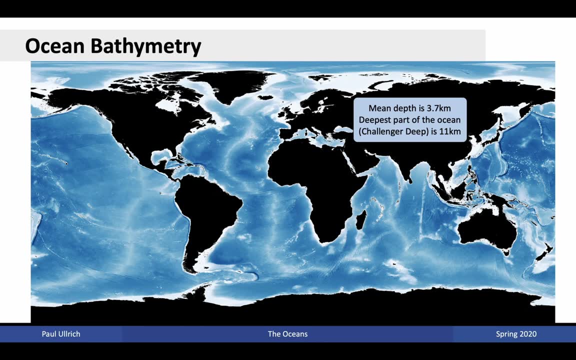 through this top 200 meters or so. Consequently, we have very homogenous properties of this ocean that occur within this boundary layer. Here's a depiction of the ocean bathymetry. The mean depth of the ocean is around 3.7 kilometers, but the deepest part of the ocean is about 30-45 degrees. The water flow is: 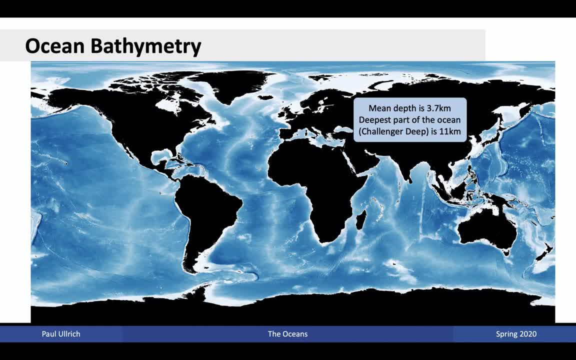 is the Challenger Deep at approximately 11 kilometers depth Throughout the ocean. you see that there is pretty significant variations in topography. In particular, pay attention to the Atlantic Ocean in the North Atlantic and the South Atlantic, where the Mid-Atlantic Ridge of course, provides a effectively mountain range that goes through the center of the oceans. However, elsewhere, 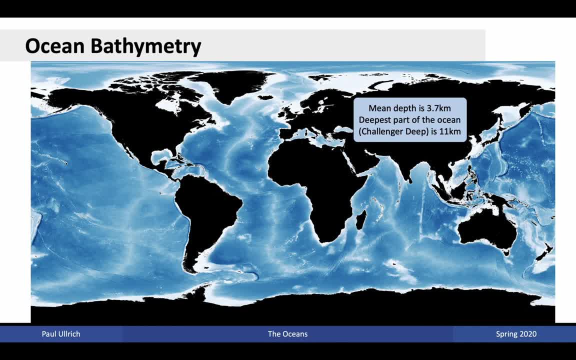 we can see evidence of these ridges. These are large-scale tectonically driven features that are responsible for producing very rough topographic variation within these oceans. Because of a lack of weathering, that is, because the ocean doesn't experience rainfall, we have 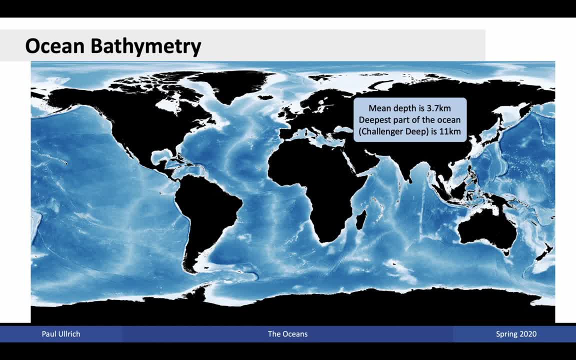 typically that in the oceans you have much rougher bottom topography. The bottom topography in the oceans is referred to as the bathymetry and, as I mentioned, it tends to be much rougher along the bottom of the oceans than it does over the land surface. 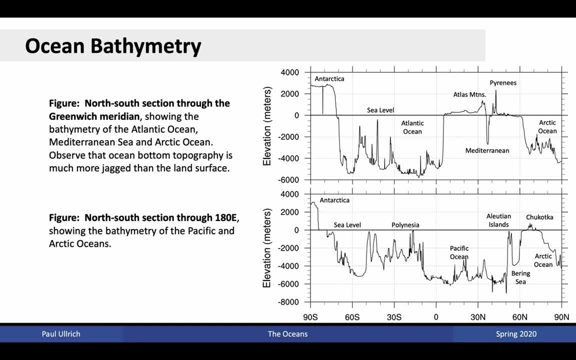 Here are two cross sections through the ocean. On the top we see a north-south section through the Greenwich Meridian that is zero degrees. On the right hand side we have the Arctic Ocean. on the left hand side we have Antarctica. As you can see, there are some pretty significant variations in topographic. 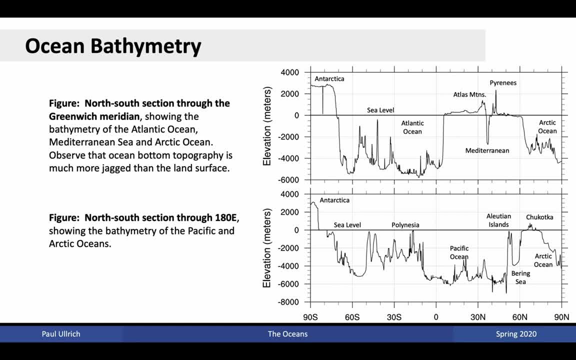 height. The land surface represents only a small perturbation above sea level, whereas the ocean depth extends quite deep. in this image You'll also see again that topographic roughness at the bottom of the ocean that I'd mentioned previously. The bottom figure shows a north-south section through 180 degrees east, much of which is 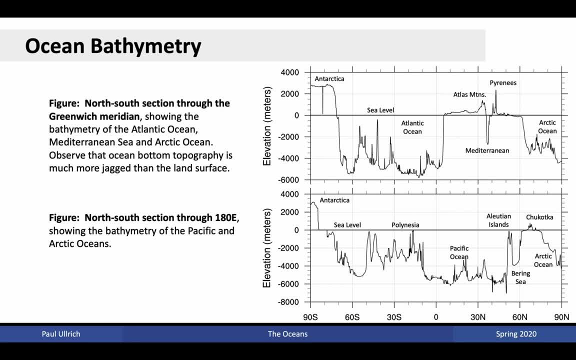 underwater Again. the oceans of the world are approximately 70% of the total earth's surface area, so it's not unexpected that we would be able to take large cross sections and find almost into the entirety of the cross section underwater. What I want you to observe here is that there is significant variation in this underwater topography. 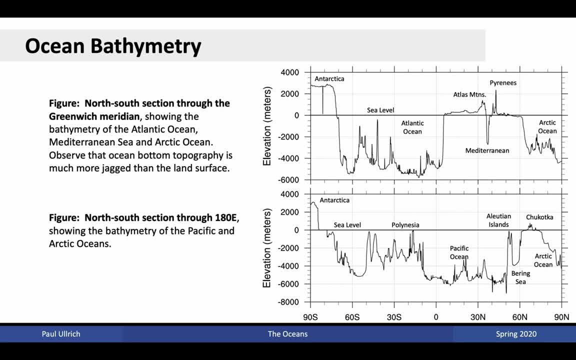 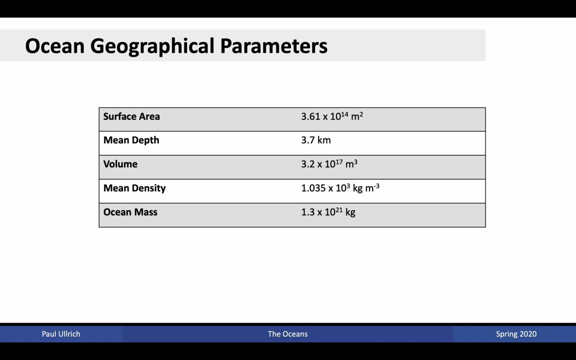 and since it is a solid lateral boundary to the oceans, that is, it's an impervious, permeable boundary- you can have significant effects that are driven by this underlying topography in terms of the underlying ocean dynamics. All right, there's a few geographical parameters that are important to know for this, for the ocean. 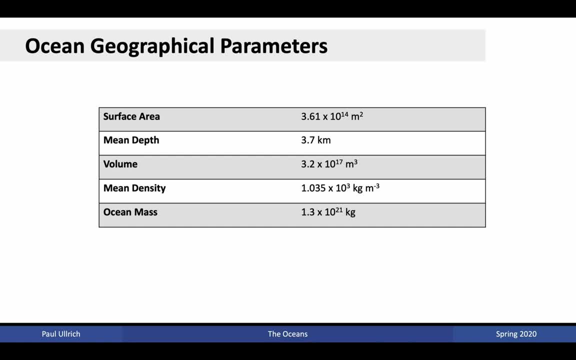 The surface area is about 3.61 times 10 to the 14 square meters. mean depth, again 3.7 kilometers. total volume of the ocean: 3.2 times 10 to the 17 cubic meters, the mean density of the ocean, which is going to be important when we assess variations of that density. 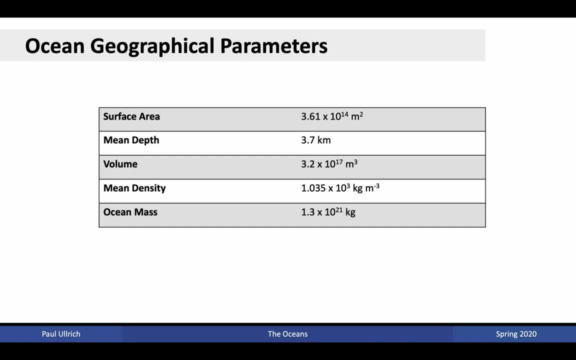 because, through the equation of state, is about 1.035 times 10 to the 3 kilograms per meter cubed and the total ocean mass then is about 1.3 times 10 to the 21 kilograms, The physical parameters associated with the ocean which are important for 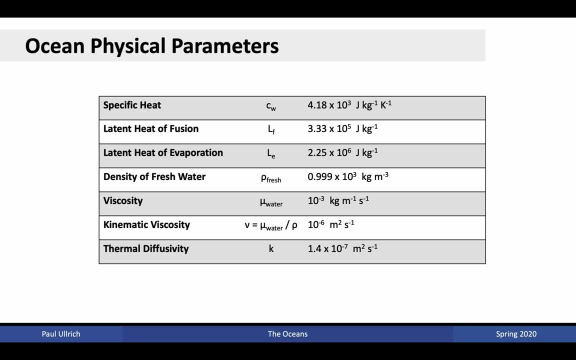 understanding things like heat capacity, as well as evaporation and condensation, include the specific heat of water at 4.18 times 10 to the 3 joules per kilogram kelvin, latent heat of fusion at 3.33 times 10 to the 5 joules per kilogram, and latent heat of 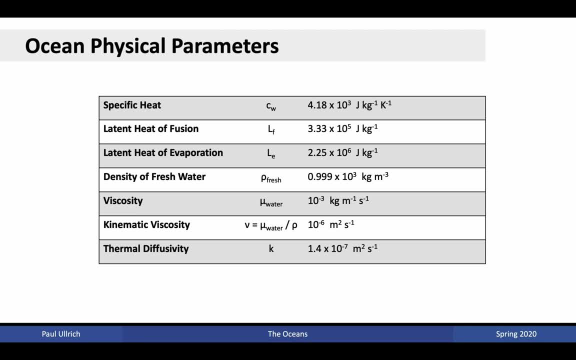 evaporation at 2.25 times 10 to the 6 joules per kilogram. The density of fresh water is about a thousand kilograms per meter cubed. Note that this is pretty different than what we saw on the previous slide with regards to the density. average oceanic density of 1.035 times 10 to the 3. 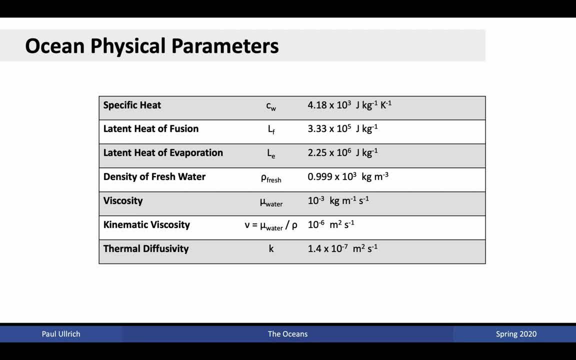 kilograms per meter cubed, and much of that difference is again because we have salinity in the ocean. The viscosity of the water is about 10 to the minus 3 kilograms per meter per second. this is a fairly small quantity and consequently it means that the viscosity doesn't play a huge. 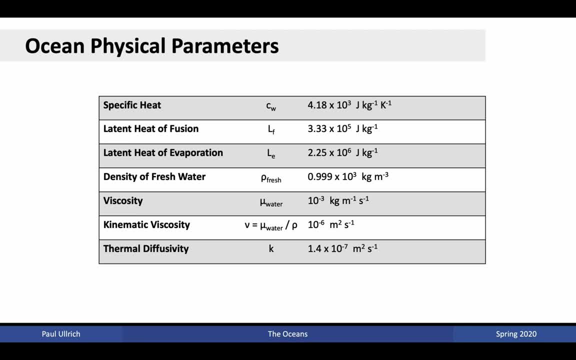 role in affecting the ocean dynamics, except in regions where friction is important So much like in the atmosphere, where we found friction is important in the near surface layer. analogously, in the ocean, friction is primarily important in the mixed layer, near where the atmosphere and 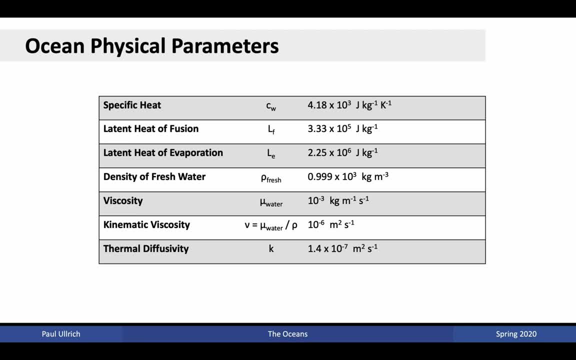 ocean meet and in the near surface layer. friction is important in the mixed layer and at the lateral boundaries, where the oceans meet the continent. The thermal diffusivity of the ocean is about 1.4 times 10 to the minus 7. 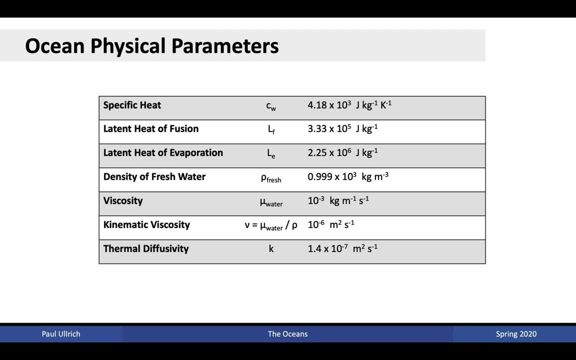 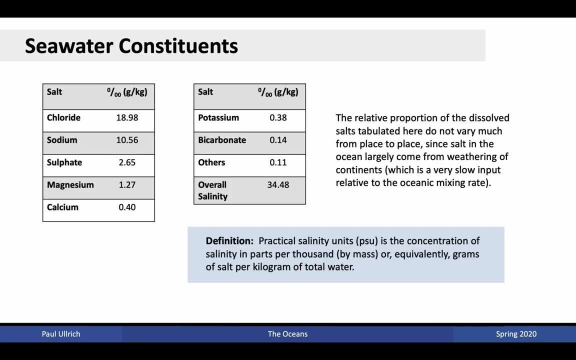 meters squared per second. Again, these quantities may be useful in coursework or in doing a deeper quantitative analysis of the oceans. All right, the salinity of the ocean of course plays a big role in the overall physical character of the ocean. Here we have listed the 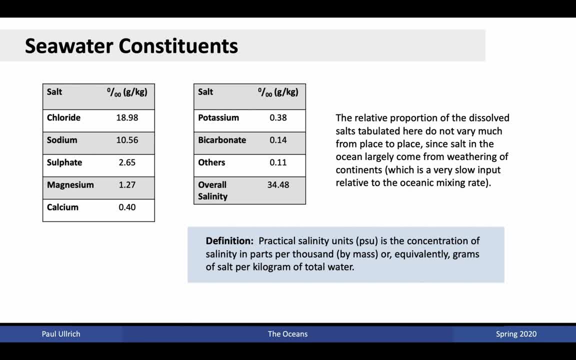 two primary contributors to that salinity, The most important contributor being chloride and the second most important contributor being sodium. So the combination sodium- chloride, which you may know as table salt, is pretty much the main contributor to sea water and consequently, why evaporating sea water can then provide you with an easy source of table salt. 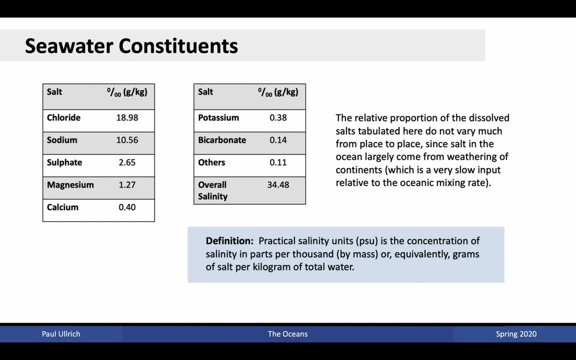 However, there's other contributions as well to the salinity of the oceans, including sulfate, magnesium, calcium, potassium and carbon dioxide. mundane natriure and awagenite came in an equivalent one. PropCola死are and glacial racism- see when burned oxygen. Narr рос in C3т and was engaged Ana tremendously in both sources. Models were many times exhausted and could have by water tank etc. Telka terinsky also consume these solutions In many 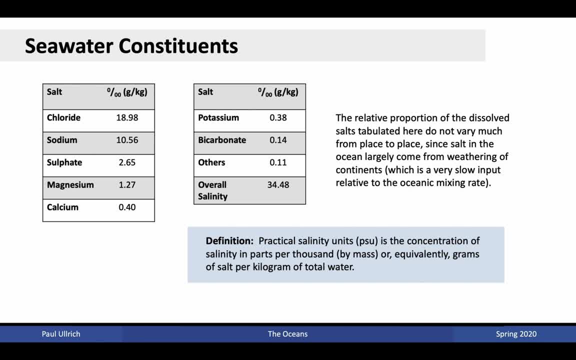 potassium and bicarbonate. The others then make a relatively small contribution to the overall salinity, But in terms of grams per kilogram, the salinity is about 34.48 grams per kilogram. Note that if you take this and add it to the density of freshwater, you'll 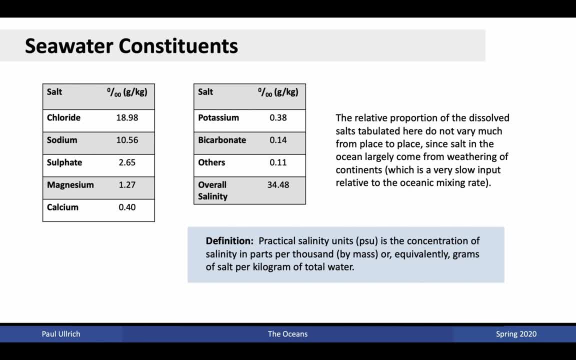 find that you'll get basically the average density of ocean water Alright. so the relative proportion of the dissolved salts don't vary too much from place to place, although different ocean basins do have certain preferences for different salts. But most of it comes essentially from weathering of the continents. So whenever 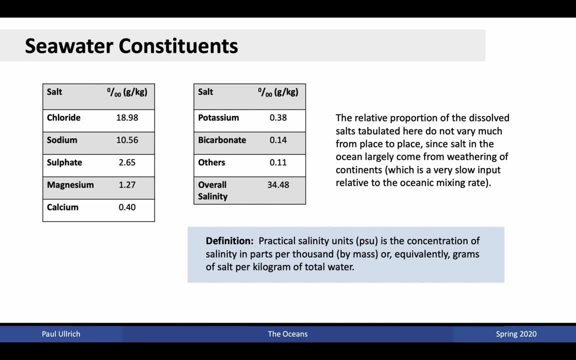 we have a rain event, for instance, on the continents, that can wash some minerals into the rivers, which can then eventually get washed out into the oceans. That washing out then provides a source of these salty constituents to the oceans. The deposition time or how? 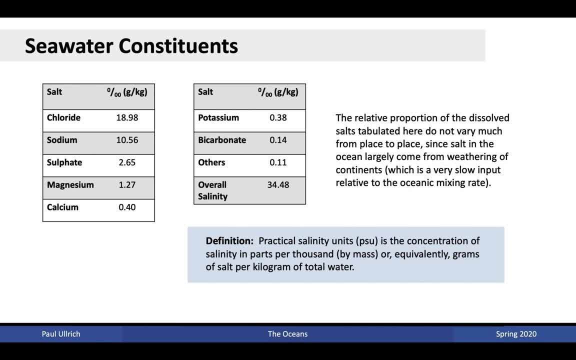 long it takes for the salts to basically turn into solids within the ocean occurs over a very short period of time. So that's a lot of salt, And so, basically, the system has ended up in essentially a quasi-equilibrium, where the inputs from rivers is balanced by the sedimentation of salts within the oceans, So source equals. 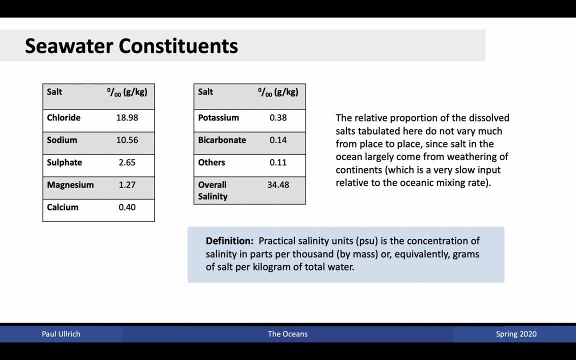 sink. The quantity that we're going to need to use in order to measure the salinity of the oceans is known as the Practical Salinity Unit, or the PSU for short, And it's the concentration of salinity that we're going to need to measure the salinity of the oceans. So the 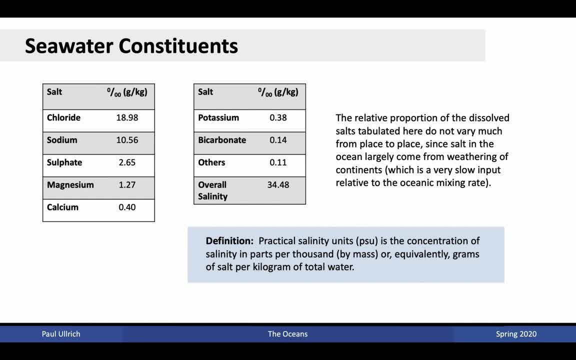 salinity of the oceans can be in, basically, parts per thousand by mass, or equivalently grams of salt per kilogram of total water. So not a particularly obscure unit to deal with, but one to keep in mind as we go through our analysis. 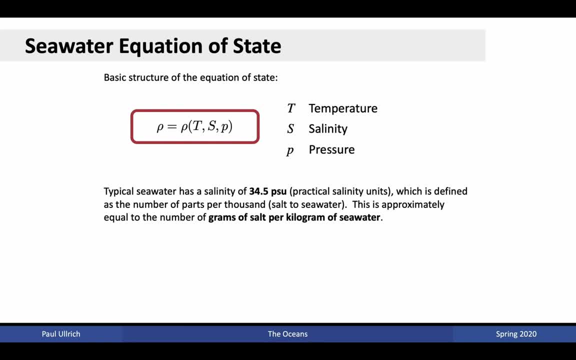 All right, let's talk about the equation of state associated with seawater, since that is important in determining the thermodynamics and then, consequently, the dynamics of the ocean. The basic structure of the equation of state is that the ocean is a very large ocean and that the temperature, salinity and pressure at that location is a function. 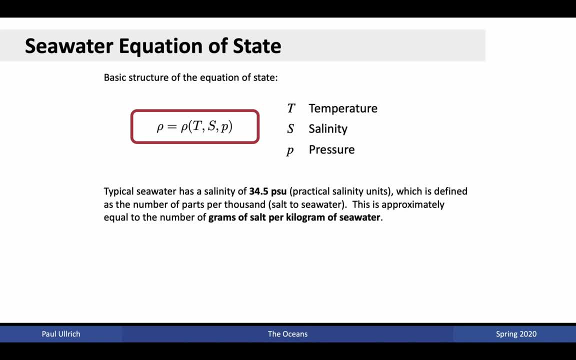 of the density at a particular location. Compare this, for instance, to the equation of state for the atmosphere, which, you may recall, is exactly the ideal gas law, which equates the pressure to the density times, the ideal gas constant times the temperature In the oceans. 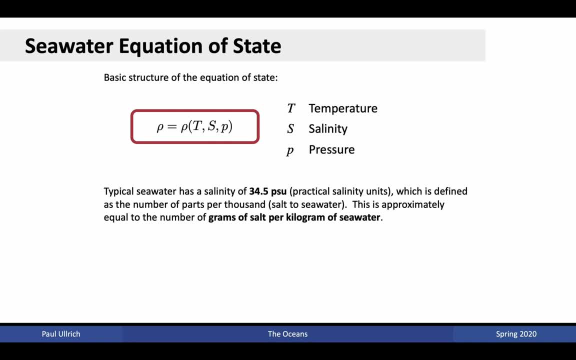 the equation of state tends to be a little bit more complicated than that and we'll go into some details about that shortly. The baseline salinity of the oceans is about 34.5 practical salinity units. That will be important in a moment. 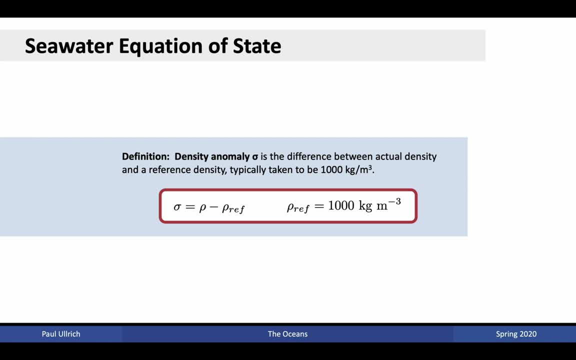 In order to assess the density. it's typical to not use the density directly in expressing this equation of state, but instead use the density anomaly, which we use the Greek symbol sigma to denote. This is the difference between the actual density and a reference density. 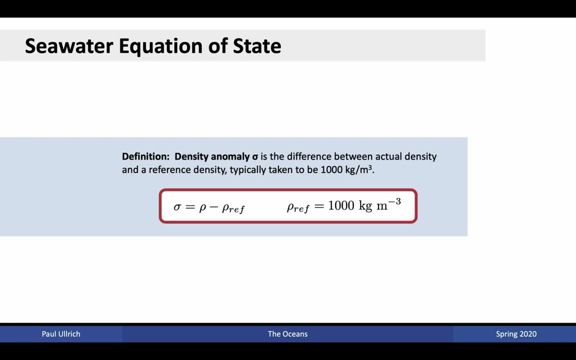 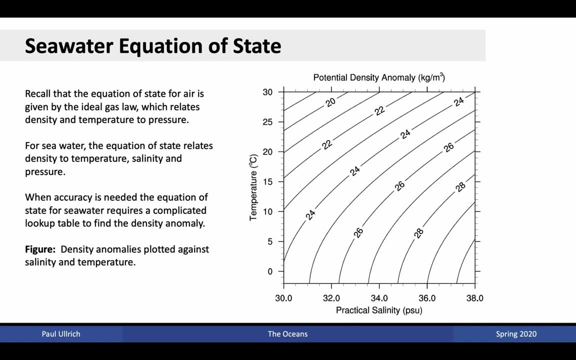 typically taken to be about a thousand kilograms per meter cubed, or approximately the density of fresh water. The equation of state of air is again given by the ideal gas law, which relates density and temperature to pressure. However, this simple relationship doesn't quite hold, for 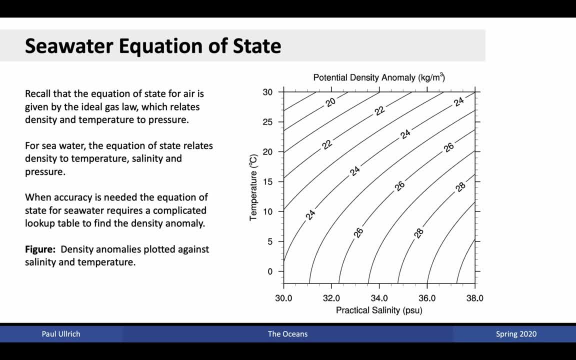 ocean water and the actual expression that describes the equation of state with ocean water can get quite complicated. Consequently, it's typical to actually express this equation of state in an empirical manner, that is, We can plot the equation of state with the equation of state with the equation. 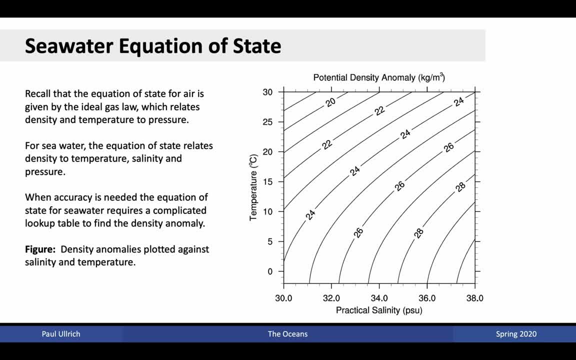 of state. In this example, we can use the density anomaly for every combination of salinity and temperature and produce a plot analogous to the one over here on the right-hand side. However, that's not very useful if we want an equation associated with the equation of state. There are various 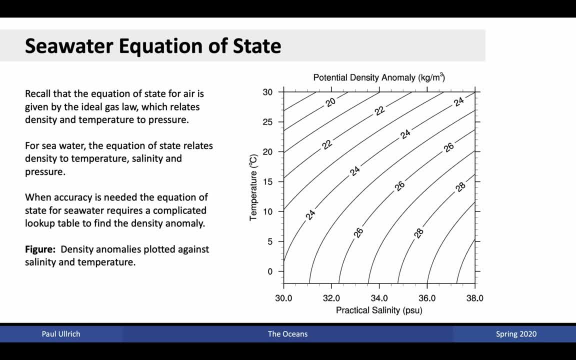 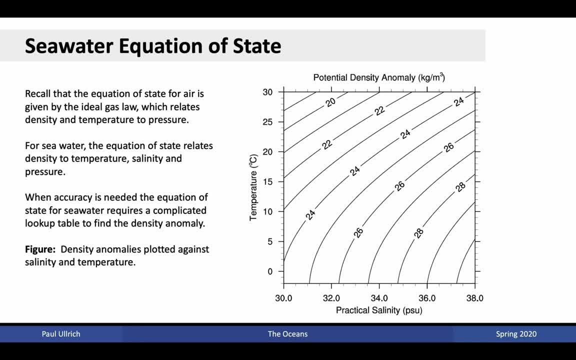 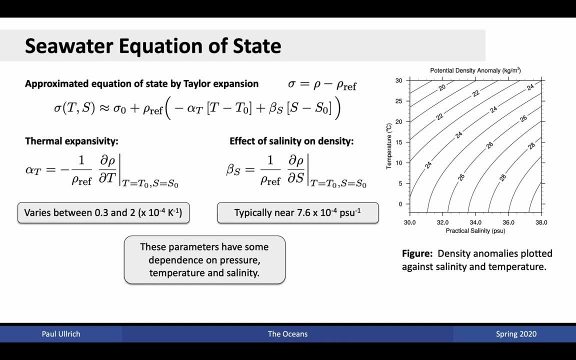 of the ocean, So the more complicated relationships can of course, be relied upon. The very simple method we're going to use for this equation of state is basically just involve a Taylor-series expansion about a particular reference temperature and a particular reference salinity. We're not going to consider pressure in our equation of state at present. 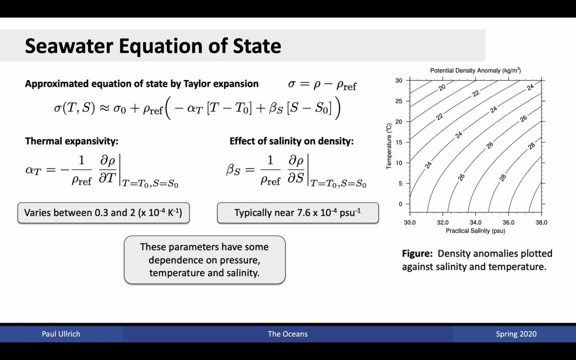 but it does play an important role when you consider differences across depth. Since our focus is primarily on horizontal dynamics at a fairly high level, we're not going to focus on depth and depth alone. We're going to consider researcher-level movement over fixed depth. That's not going to enter into this current relationship. that will be used for the 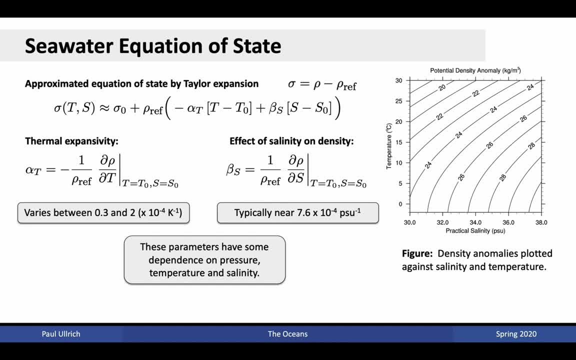 remainder of the class. So via simple Taylor series expansion, we have that the density anomaly as a function of temperature and salinity can be expressed as a base density anomaly sigma naught, plus some coefficients, times the distance between the actual observed temperature and the 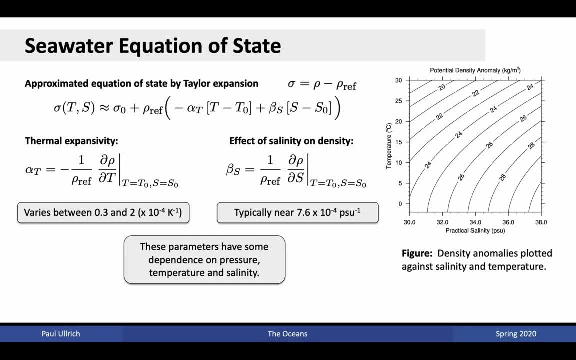 reference temperature t naught and another coefficient times the salinity minus the reference salinity, And these coefficients can then be determined empirically. Typical values for the thermal expansivity, which is this alpha parameter in this relationship, are between 0.3. 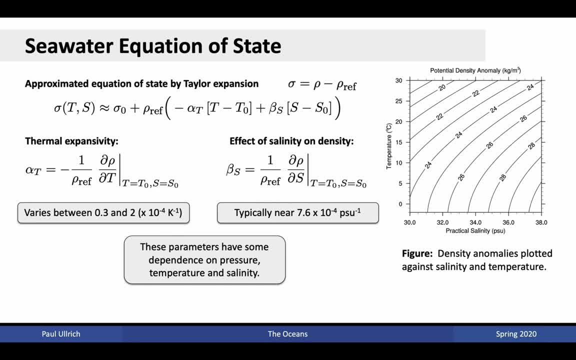 and 2 times 10 to the minus 4, 1 over kelvin, And the salinity effects are typically around 7.6 times 10 to the minus 4, 1 over practical salinity unit. So these parameters. 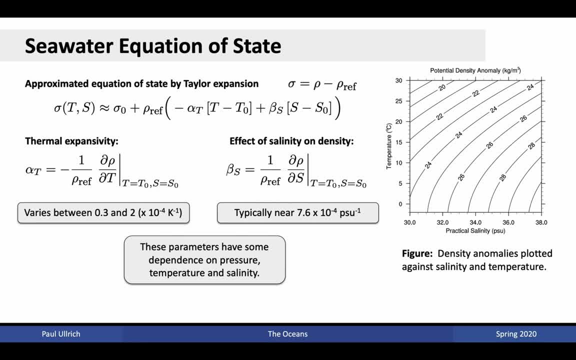 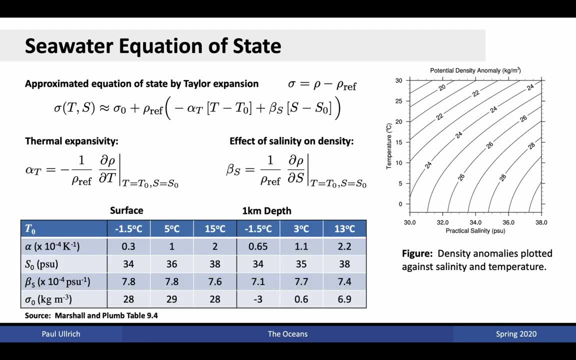 too, have some dependence on both temperature, pressure and salinity. So there's some nonlinear terms that would come up in a more complicated expansion, But for the time being we can use this as a good approximation to the equation of state, and it provides all we need for our 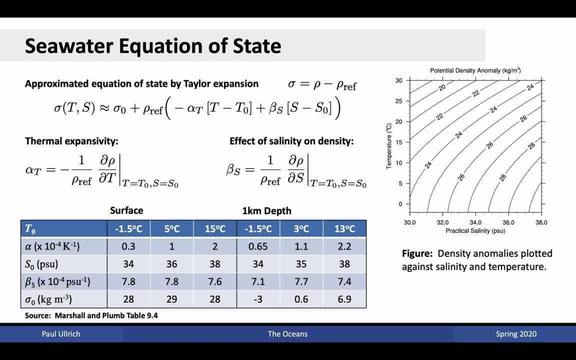 purposes. Here is a reference table. On the left-hand side we see the various parameters that must go into this equation of state, And we can see then for six different potential oceanic regions. we have the surface at temperatures of minus 1.5 degrees Celsius, 5 degrees Celsius and 15 degrees Celsius, and at one kilometer. 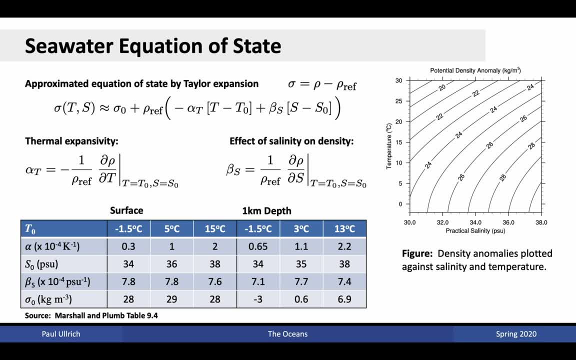 depth at minus 1.5 degrees Celsius, 3 degrees Celsius and 13 degrees Celsius. This table is taken pretty much directly out of Marshall and Plum. It's in table 9.4.. So what we can see again is that this thermal expansivity parameter tends to vary between about 0.3. 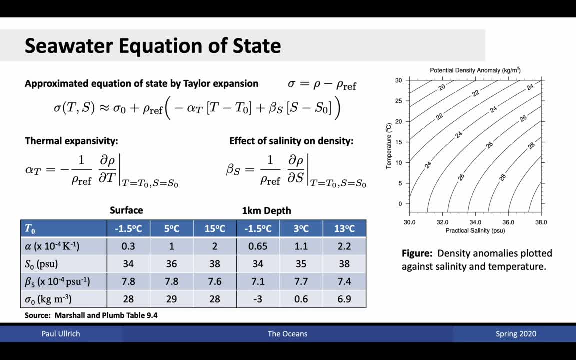 to about 2.2, tends to become larger at larger temperatures and it tends to become larger at higher pressures. The beta parameter, which is the effect of salinity on density, tends to be about 7.6 to 7.8 in the near surface and 7.1 to 7.7 at one kilometer depth There. is some temperature dependence associated with it, but it's much less of a problem. So we can see here that the surface at 1.5 degrees Celsius and 7.1 to 7.7 at one kilometer depth. There is some temperature dependence associated with it, but it's much less of. 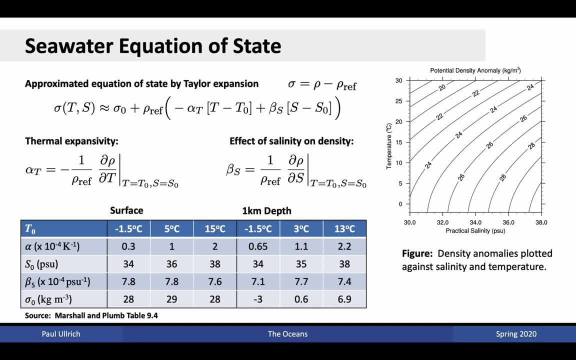 a problem. So we can see here that the surface at 1.5 degrees Celsius and 7.7 at one kilometer depth is much smaller than the temperature dependence in the thermal expansivity parameter. What is important, though, is that, for whatever equation of state you use, you make sure that 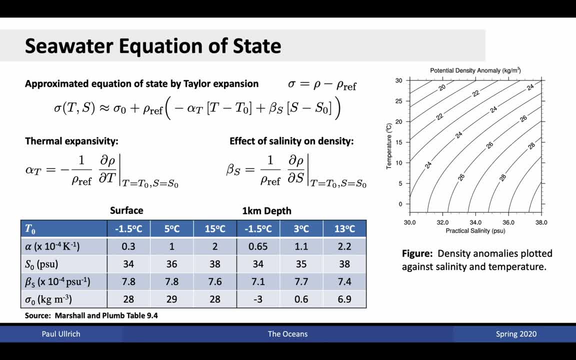 you use parameters that are appropriate for that particular region. If you are analyzing the equation of state of ocean water near Antarctica, you definitely want to use an appropriate temperature, That is, you probably want to use something closer to minus 1.5 degrees Celsius. If you're analyzing ocean temperatures in the subtropics, you want to. 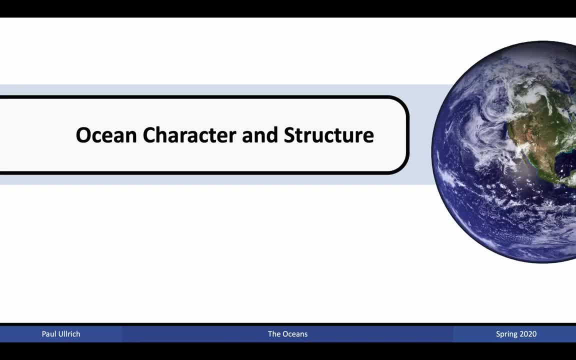 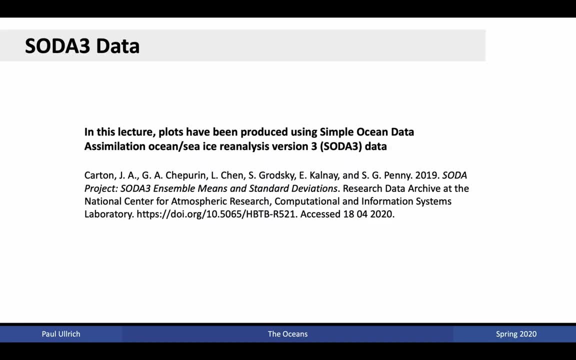 use, probably a higher temperature. All right, let's take this information, then, and look at the character and structure of the ocean. In this lecture, plots have been produced primarily using the simple ocean data assimilation Ocean-Sea Ice Reanalysis Version 3, SOTA 3 as it's known. Here's: 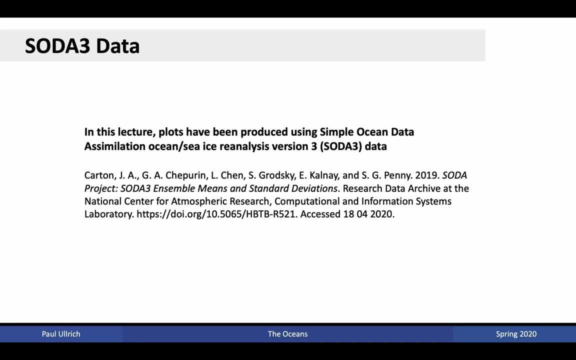 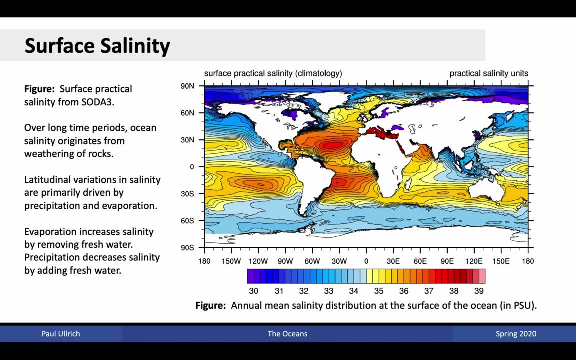 the reference associated with that. It's also available on the National Center for Atmospheric Research Research Data Archive. All right, here's a plot of surface salinity, That is, how much salt is dissolved within the surface ocean waters, As I mentioned, 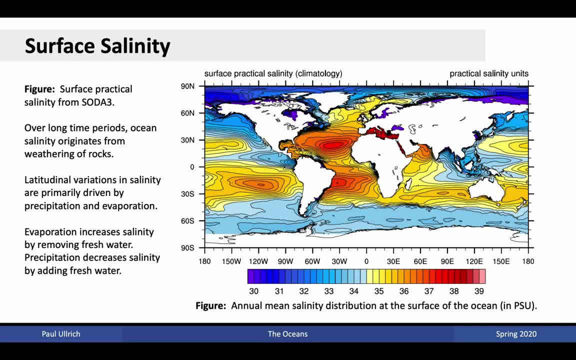 the average value is about 35 PSU. However, it varies quite dramatically depending on location. Typically, the Atlantic Ocean tends to be more saline than the Pacific Ocean and the Indian Ocean, And, in particular, the Mediterranean Sea, is notorious for being very saline compared. 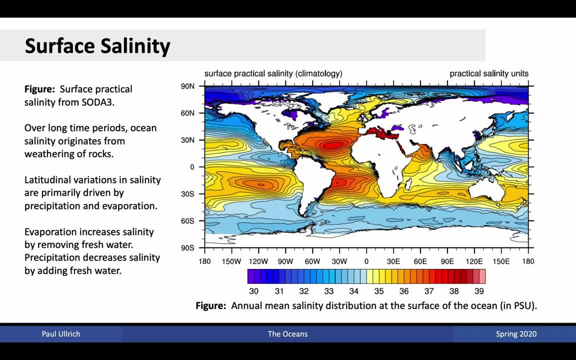 to either of these ocean basins, Whereas at northern latitudes we see instead that the ocean water tends to be more saline than the Pacific Ocean, and the Indian Ocean tends to be not particularly saline at all, That is, there's very little dissolved salt content. 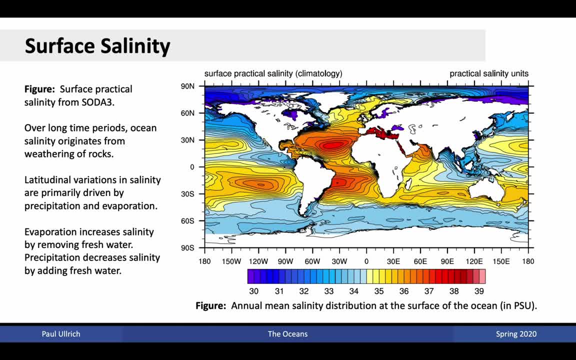 It's worth noting that, since the density of the ocean water is driven up by the salinity content, we of course have that. the Atlantic Ocean waters then tend to be more dense in general. The distribution of the salinity is also very interesting within each ocean. 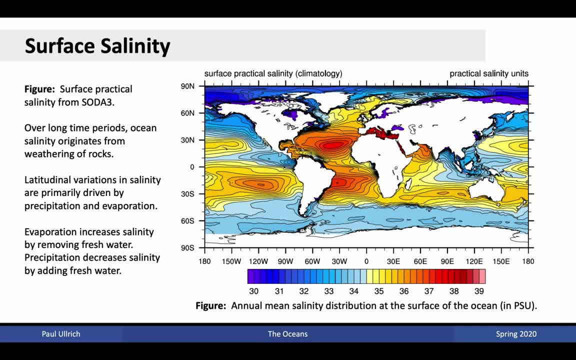 basin. Actually, we see that in the subtropics regions of both the northern hemisphere and the south hemisphere the salinity of the ocean water tends to be more saline than the salinity of the southern hemisphere. We tend to have concentrated blobs of salinity with 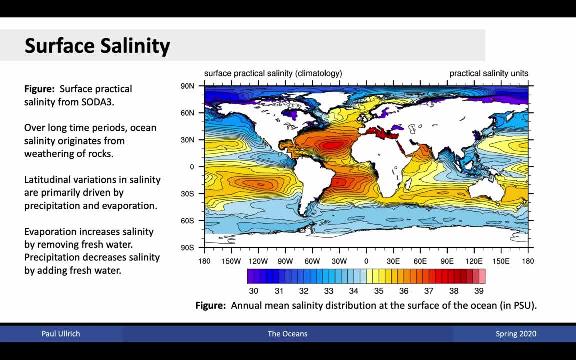 some of the highest salinities then showing up at about 30 degrees north and 30 degrees south. The equator, on the other hand, shows fairly low salinities, In fact, if one was to compare this plot with, for instance, the surface pressure plot that we saw last time. 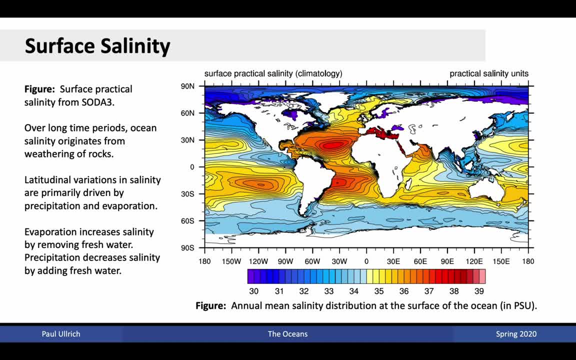 you would notice that there seems to be a close correspondence between these two. In fact there is a relationship going on here. Recall that in regions of low pressure we have convective activity that is more saline than the salinity of the ocean water. So in fact there is a. 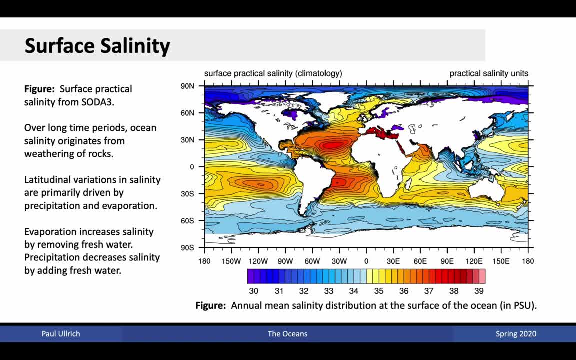 close correspondence between these two. In regions of high pressure, we have suppressed precipitation because of subsiding air. This precipitation ends up being the primary driver responsible for then inducing changes in surface salinity, Namely, injections of fresh water from precipitation around the intertropical convergence zone is responsible for driving down the average. 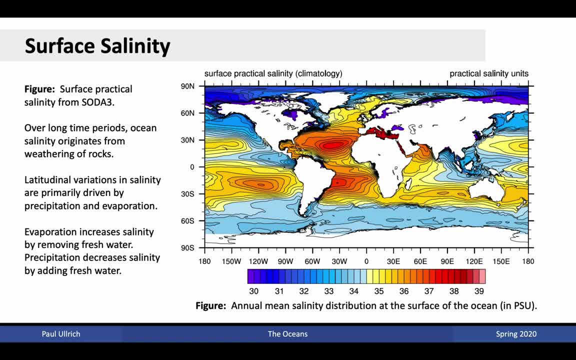 salt content in this region, whereas evaporation that occurs in regions of subsidence, where precipitation is subsiding, is responsible for driving down the average salt content in this region. So the temperature that is suppressed is responsible for taking fresh water out of the seawater, leaving more saline water behind. So these two factors together, then. 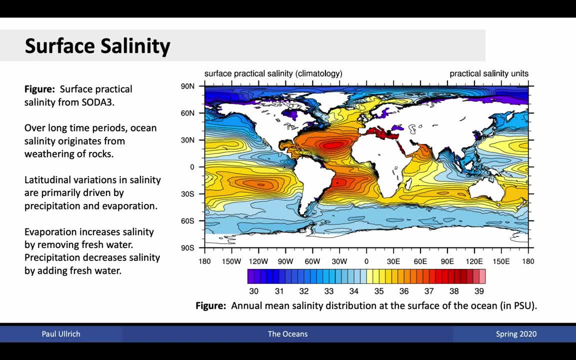 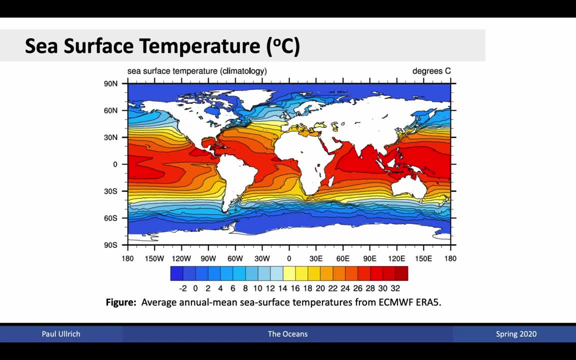 are responsible for driving these major patterns in the ocean basins. Alright, here's a plot of sea surface temperatures. Sea surface temperatures are, perhaps unsurprisingly, not particularly different than the near surface temperatures that we've seen in our previous analysis. However, what is worth emphasizing here is that temperature is not 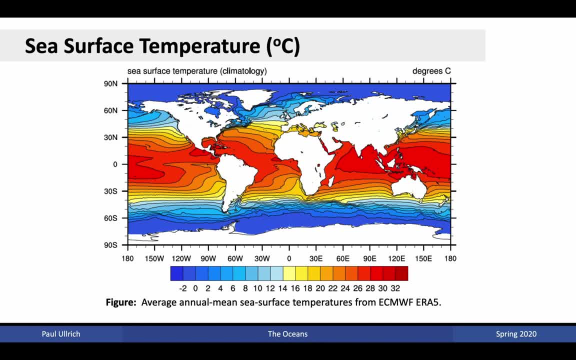 a matter of a matter of fact. In this analysis, we see that the sea surface temperatures are different. The ratio of sleep and concentration of water between the sea surface temperatures and the sea surface temperatures actually are not the same. While the pressure dropped below 0 degrees in the polar regions, the sea surface temperatures are then. lower than the Ice pull temperatures, and those temperatures are also covered with sea ice over the corresponding winter season. That sea ice then provides an insulating layer for seawater underneath. Temperatures can actually drop below 0 in these regions, while the water remains liquid. because, of course, seawater, with its extra saline dahlias, actually requires a layer of water to eliminate the sea water layer, and so the seawater can actually cause the seawater to drop below zero in these regions. So this is a really interesting. trying to bring out just a little bit of 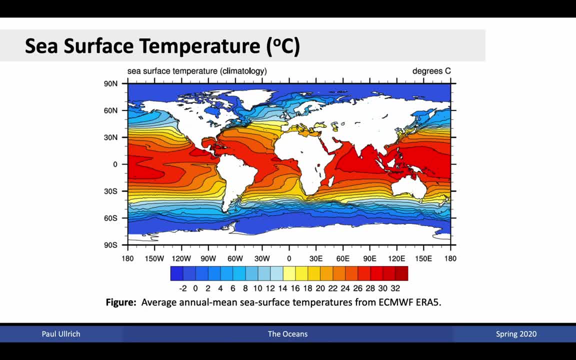 extra saline content has a much lower freezing temperature than fresh water. Other variations here include clear differences that occur along the western and eastern coasts of these continents. Pay close attention to the western coasts, where we see perhaps an enhancement of the temperatures that are. 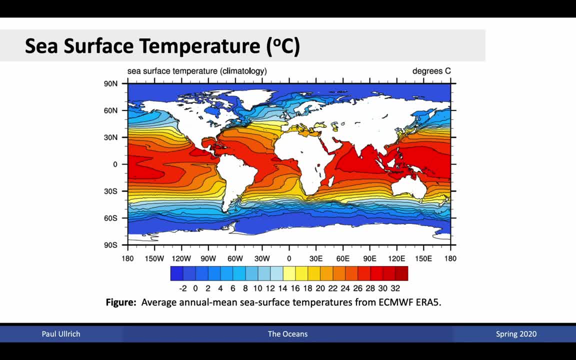 drawn northwards because of strong western boundary currents and along the east coast, where we see cooler temperatures pushed south in these ocean basins. This is again part of the general circulation of the overall ocean system We also see because of the lateral boundaries produced by the continents. 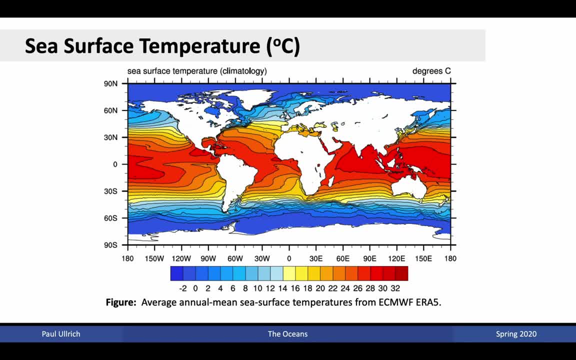 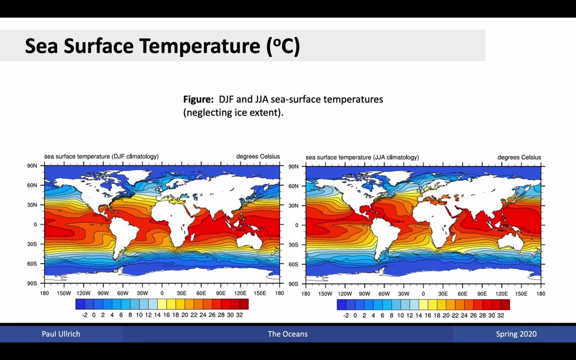 that we have some variations in the sea surface temperatures because of how those ocean waters are actually moving around in these regions and we'll investigate that in a bit more detail later, once we get into ocean currents. Here are the seasonal variations in sea surface temperatures On the left-hand. 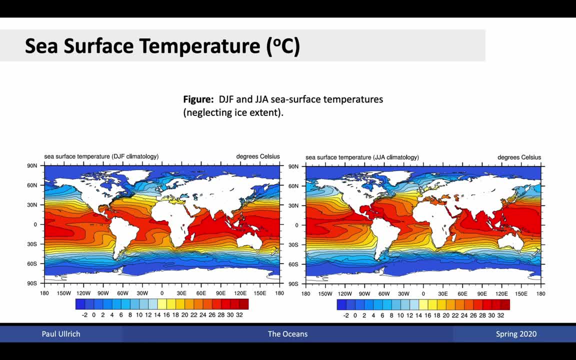 side we have the December-January climatology, or the Northern Hemisphere winter season climatology, and on the right-hand side we have the June-July-August climatology. You'll notice perhaps initially that the temperature difference between these two is not particularly large. that is the same large-scale pattern is essentially. 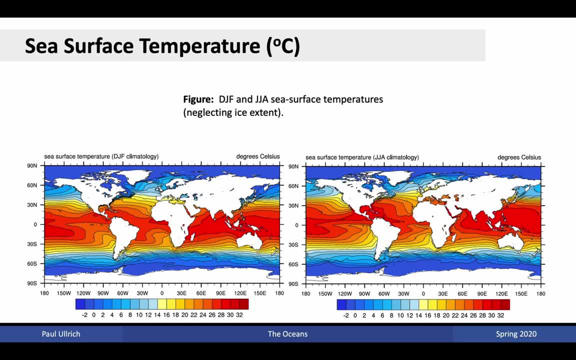 present in both plots. There are some more subtle differences in these, though, if you pay close attention. For instance, there is a small seasonality associated with the motion of ocean waters. In DJF, temperatures tend to be warmer further south or through the Southern Hemisphere, and in JJA, those temperatures tend to be 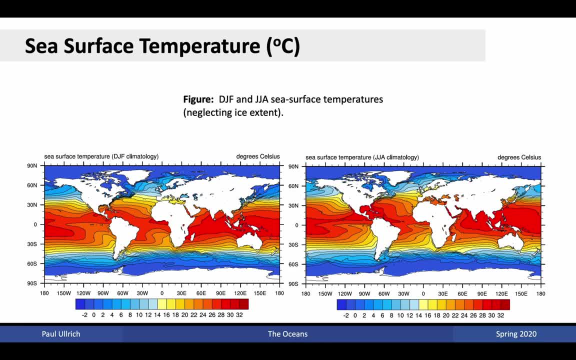 slightly warmer through the Northern Hemisphere. On inland bodies such as the Mediterranean and Black Seas, we'd see, of course, much stronger temperature dependence because there is simply less water to circulate. That thermal capacity of water plays a very important role in regulating the climate system in 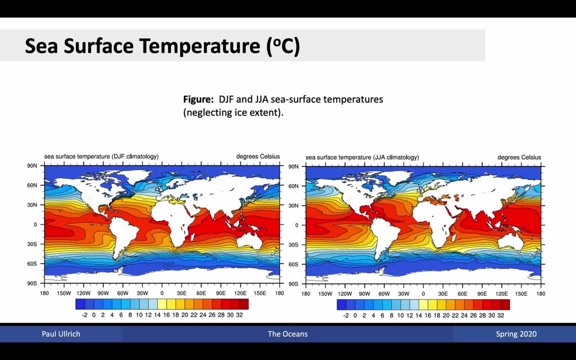 particular, because water has a large heat capacity associated with it, it is very difficult, in order to make large-scale changes or significant changes to the overall temperature pattern of the Earth's oceans. This regulating capacity is, then, very important for not only affecting the climatology of coastal communities, but also in maintaining 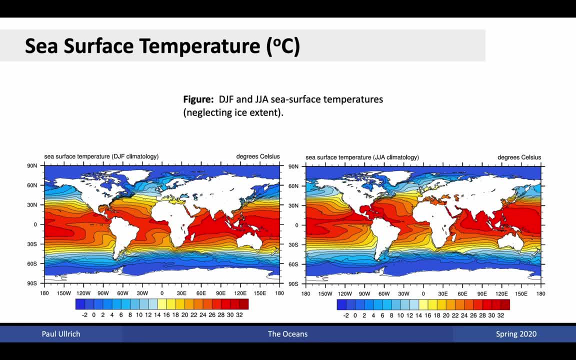 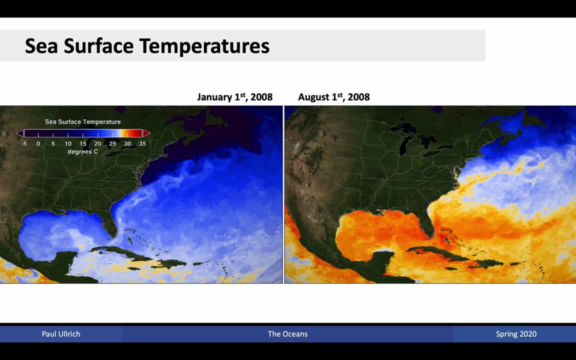 a reservoir for excess heat within the Earth's system. Here are two plots of sea surface temperatures, again showing seasonality. Here we're zooming in over North America and in particular we're pointing out a cool feature of the oceanic circulation in the Atlantic, which is 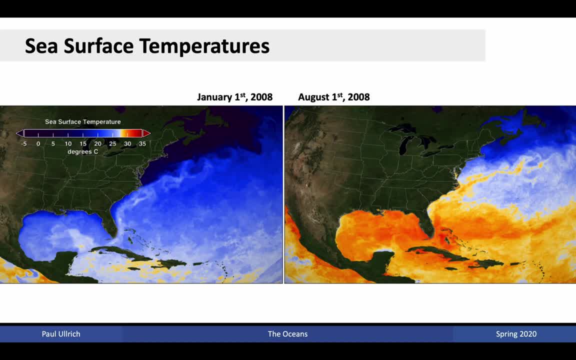 the Gulf Stream. You'll notice in particular in both the January and August pictures here that there is a sharp temperature contrast. that occurs approximately off of the coast of North Carolina and extending to the northeast through the ocean There is significant eddy activity. that also goes. 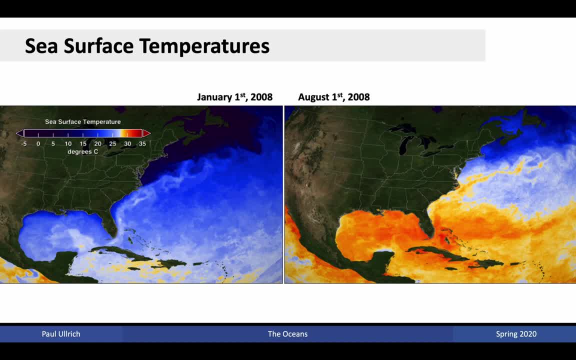 along here in the form of basically little mixing, little circles of mixing, and that's a natural feature of the oceans as well. Basically, we have these eddies that are responsible for continuously mixing ocean waters, But this thermal contrast is quite powerful and very important in adjusting the climatology of Europe, That is, warmer waters. 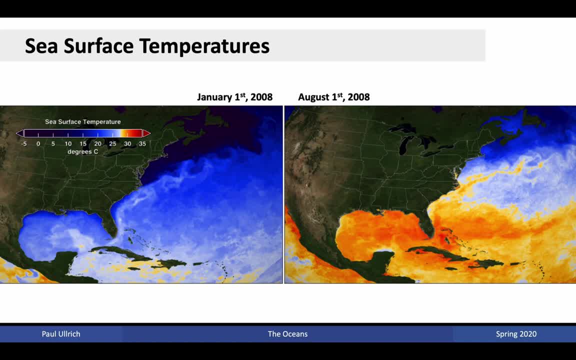 carry across the Atlantic and provide a buffer for wintertime conditions in Europe. You'll also notice that in the shallower waters of the Gulf of Mexico we have much warmer temperatures and much stronger seasonal variation between these two seasons. The warm temperatures in particular that occur within the Gulf of Mexico from August through December are responsible. 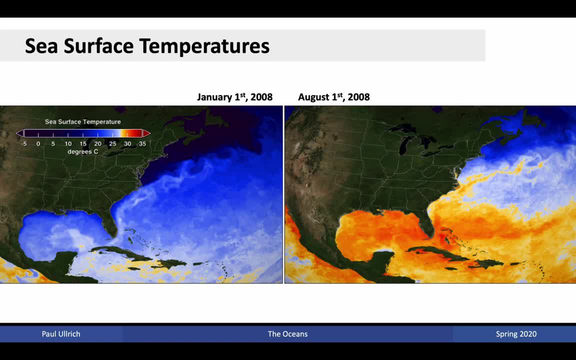 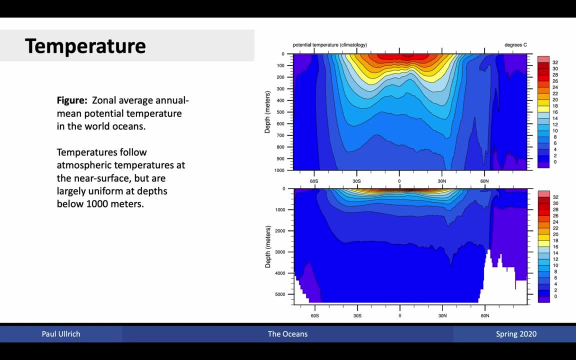 for driving much of the Atlantic hurricane season and what makes basically this southern region of the US so susceptible to strong hurricanes. Okay, let's look at temperature in terms of a zonal cross-section. Here we've done a zonal average over the whole ocean. 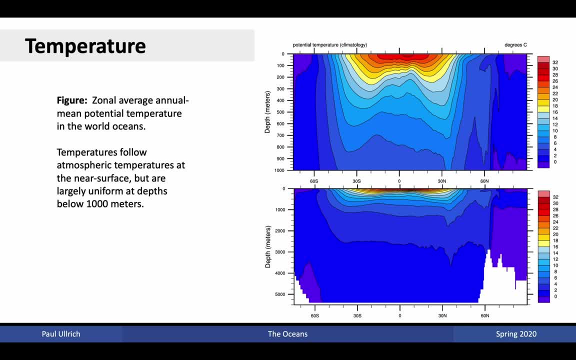 at all possible longitudes. We now take some maps that from the continent view, but the of the ocean on the right North, about 60 degrees north, we have the Arctic Ocean and you might notice in these figures that there is some significant differences in terms of the overall. 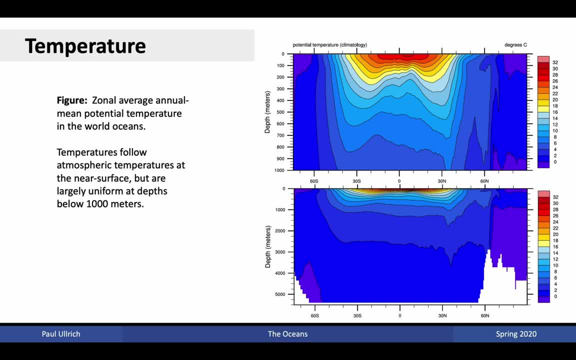 character of the ocean in that region. However, looking at the equatorial regions, we see some interesting profiles here. So in the top plot here shows the first 1000 meters of depth and the bottom plot shows that all the way down to 5,500 meters. If you focus on the top plot you'll notice that analogous to the atmosphere. 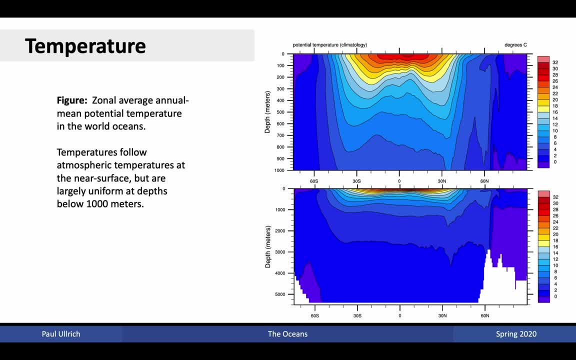 we of course have the warmest temperatures occurring at the equatorial surface and temperatures dropping as you go deeper in the ocean. Recall: the same thing happens in the troposphere As you get farther away from that equatorial surface, if you go higher up in the 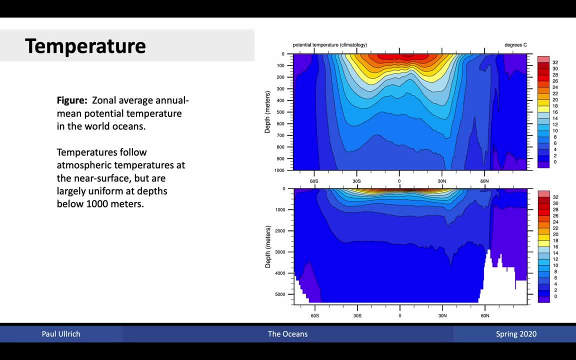 atmosphere or towards the poles, you end up with cooler temperatures. The reasons for this are largely radiative, That is, the ocean only really experiences direct radiative forcing through the near surface layer. There is, of course, about 200 meters in the top of the ocean, the so-called 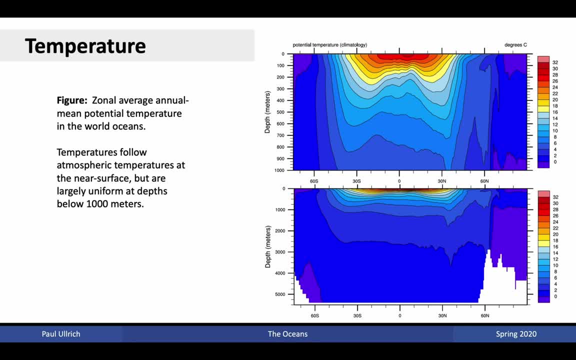 mixed layer of the ocean where we do have some homogenization because of turbulent mixing, But most of the heat is really only stuck in that topmost layer. Again, because there's very little convection, it's very difficult for the ocean waters at the near surface in order to circulate. 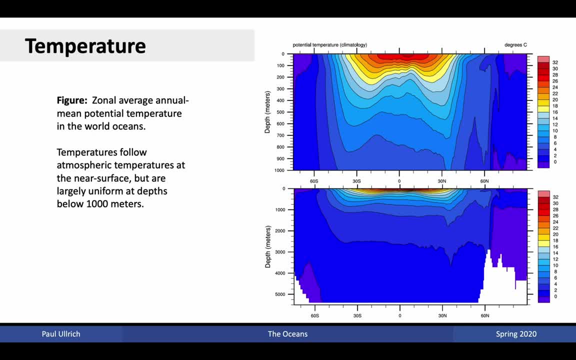 to depth. So the deeper you get, the darker it gets, Consequently, the cooler the ocean temperatures overall. However, you'll also notice that it's not a perfect lens shape, That is, we don't see a semicircle of temperatures as we go to depth, as 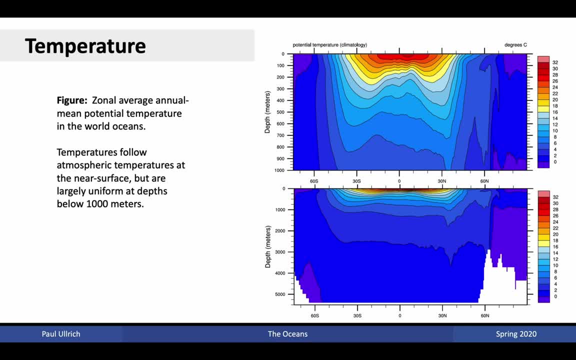 one might expect. Instead, what we see is kind of a bimodality, That is, we see the warmer temperatures at depth occurring primarily around or close to about 30 degrees north and south. We'll get into more detail about why that happens later, but 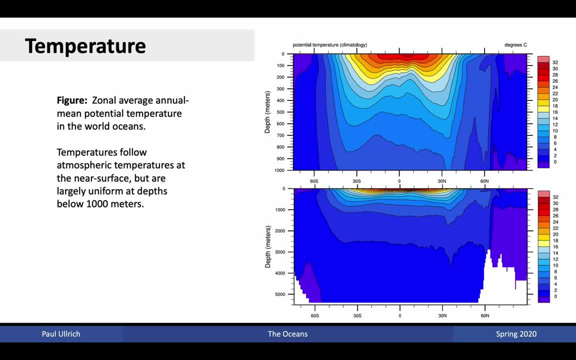 just to give you a little bit of an idea of what we're seeing, Just to give a brief spoiler, this is a region where we have more significant downwelling in the oceans, driven by Ekman pumping to depth Once we go beneath- about 1,000 meters depth in the 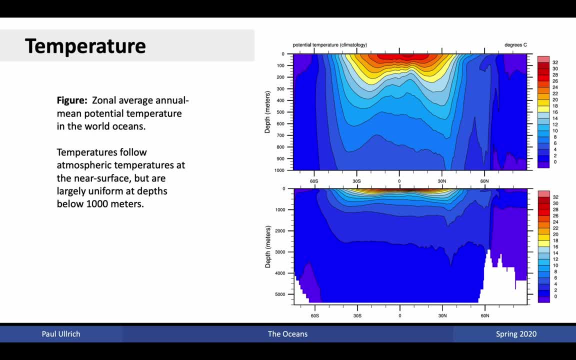 ocean temperatures are fairly homogenous And again, this is primarily because there's very little mixing that goes on down. here The ocean again tends to be fairly stable because there's no bottom warming that's responsible for driving the system away from stability. However, there 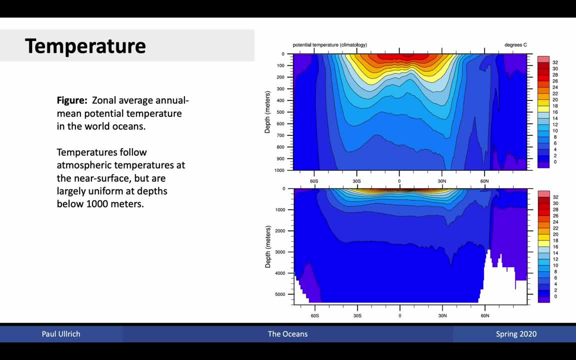 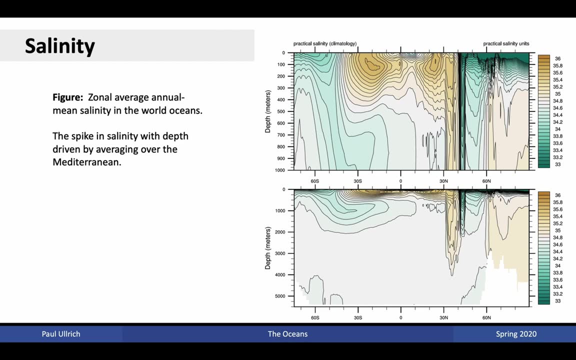 are mechanisms by which we can do that. For example, if we were to go down to the ocean, there's a little bit of a low salinityς. Then we have a region of higher salinity at about 30 degrees north and south. 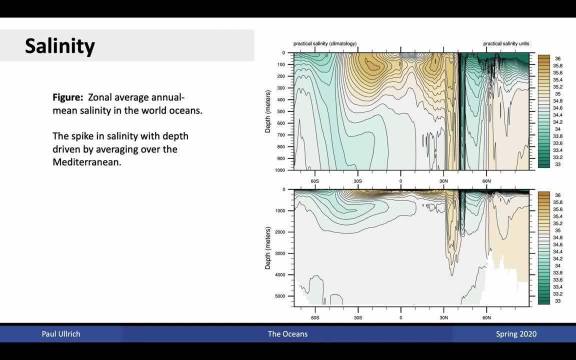 Then we have reduced salinity, particularly through the Arctic and Antarctic regions. However, there appears to be some interesting depth profile associated with this. In the equatorial regions and subtropics, we typically have a drop in salinity as you go to depth. 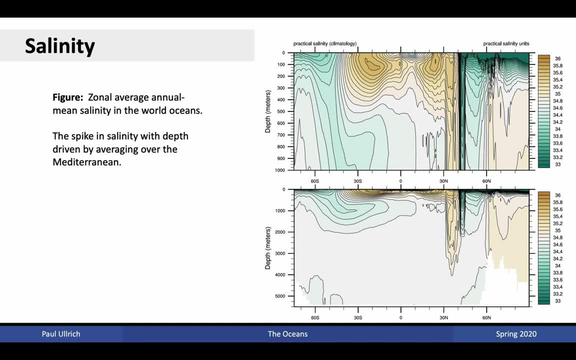 whereas in the Arctic and Antarctic regions you actually have a slight increase in salinity as you go to depth. There is also a weird peak that you might see in this diagram at just north of 30 degrees, and much of that is driven by the extraordinarily high salt content present within the Mediterranean Sea. 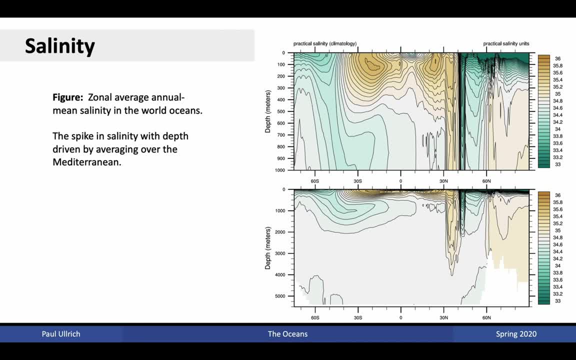 which is included in this zonal average. The overall notables from this diagram include that the maximum salinity doesn't occur right at the surface, but instead tends to occur at about 100 meters depth, whereas in the equatorial regions typically the freshest water occurs. 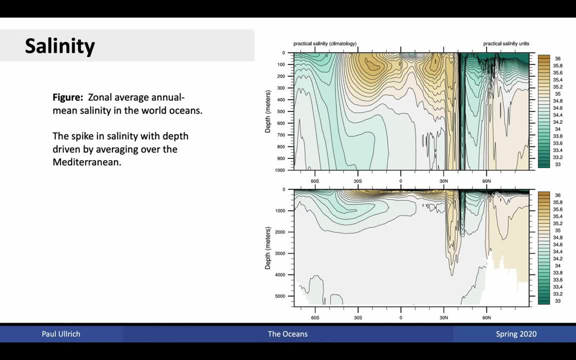 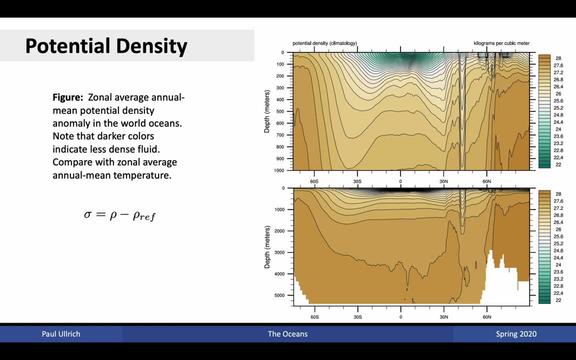 which is right at the near surface. Alright, here's the zonal mean: potential density. You might be a little bit confused at this point as to why we're plotting potential density and not real density, and the reason being mainly one of convenience. 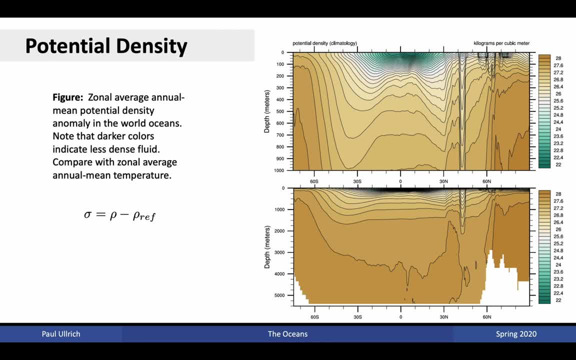 The potential density, much like potential temperature, is the density a fluid parcel in the ocean would have if brought up to a reference pressure. Thus, potential density takes into account compression effects that may be important for affecting the density of fluid parcels. However, here we're going to be a little bit sloppy and mix potential density and density. 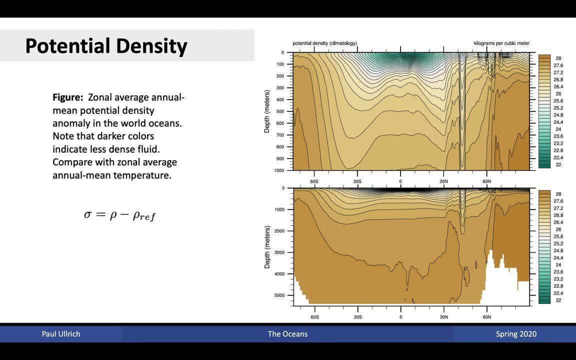 because those compressible effects tend to be fairly small, and so we're going to neglect them for the purposes of this qualitative explanation. The potential density profile that we see here looks pretty analogous to the temperature profile that we saw earlier, but you can see the characteristic spike again located here. 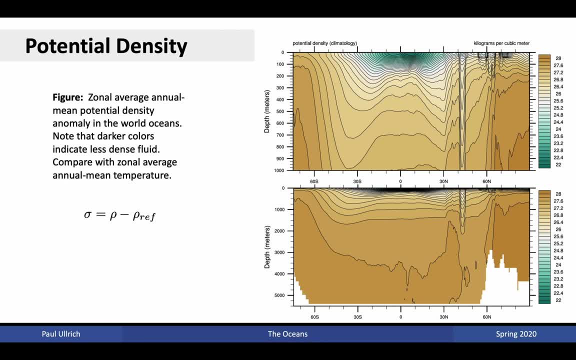 that's associated with some of the zonal averaging over some of the interior seas. The potential density profile shows its minimum value in the equatorial regions and goes towards larger values elsewhere. This is because, since potential density has such a strong dependence on temperature, 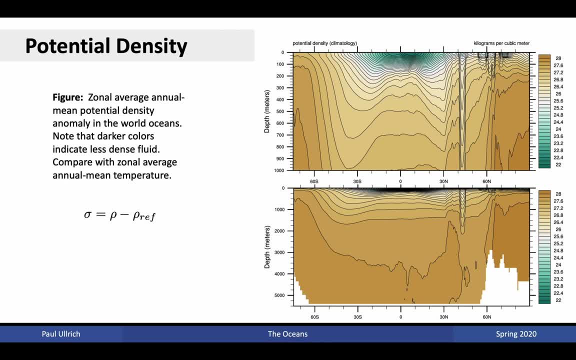 that in the warmer regions we typically have less dense fluid and in colder regions we have more dense fluid. Thus, as you move away from the warmer equatorial surface, you end up in regions that typically have more dense fluid. This is also responsible for determining the overall stability of the ocean. 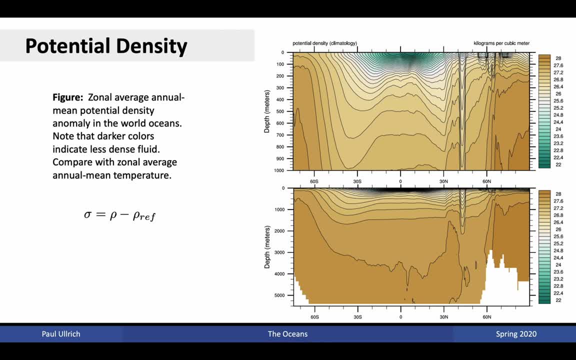 Namely in order to have a stable vertical distribution of density, what we need to have is that the potential density increases with depth. In the zonal average plot we fortunately see that throughout the oceans we have that characteristic increase in potential density as we go to depth. 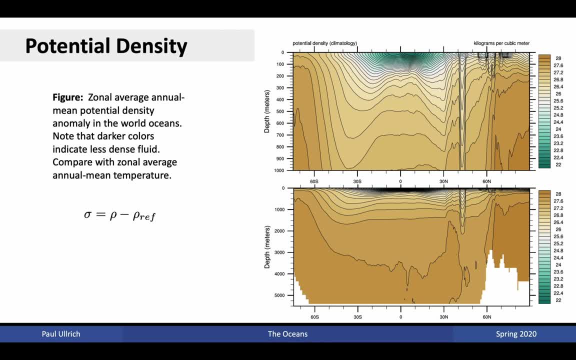 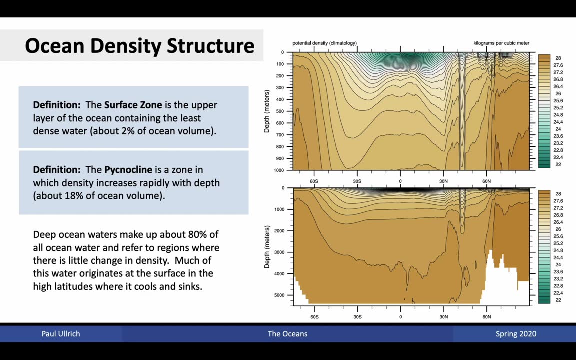 Thus, on average, we see overall stability of the ocean to convection. However, what's worth noting here is that there are aspects of both salinity and temperature that do play a role in determining the overall density structure of the oceans. Alright, the density profile can actually be used. 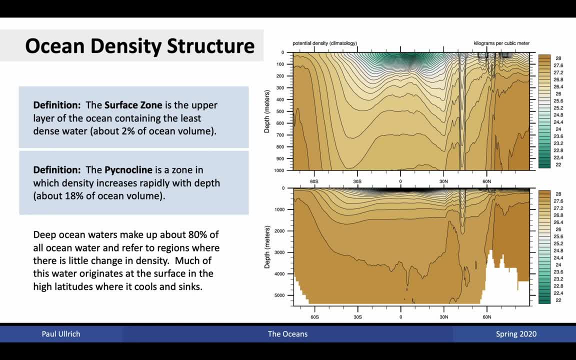 in order to define different zones of the ocean. The surface zone is typically defined as the layer of the ocean containing the least dense water, And so that doesn't include the surface zone in the polar regions, or it doesn't include the near surface in the polar regions. 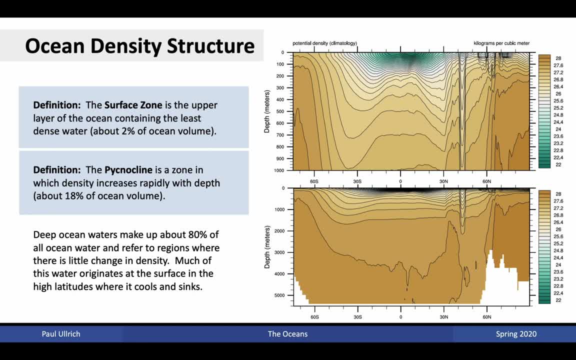 because that's where we have very dense water overall, but instead basically extends from about 50 degrees north and south through to the equator and just the near surface region of the overall oceans. This accounts for about 2% of the total ocean volume. 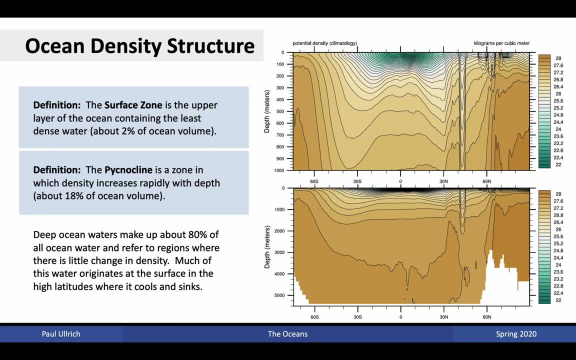 The pycnocline is a region where we have sharp variations in the density of ocean water and that's the extent immediately below that surface zone, extending down to about 1000 meters depth, below which we see essentially homogenous potential density. 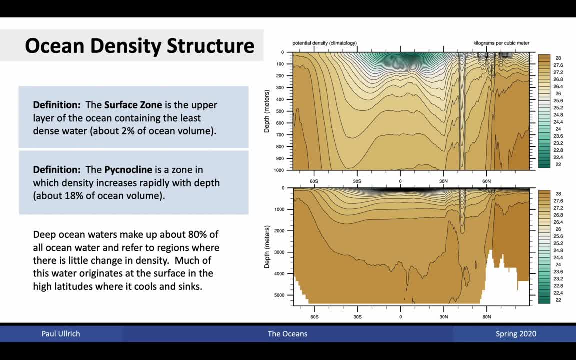 The pycnocline region corresponds to about 18% of ocean volume. The deep ocean waters, which are incredibly homogenous, typically make up about 80% of the total ocean water overall, And that includes all the ocean water that is not in the surface zone. 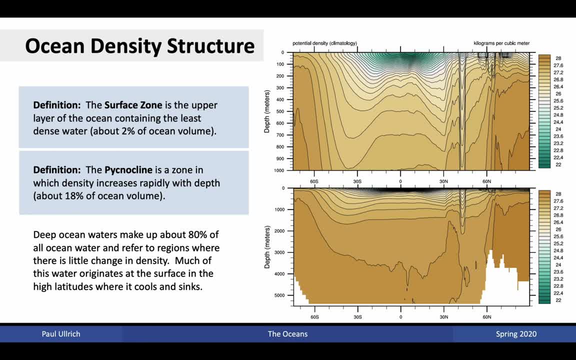 and not in the pycnocline. Much of this water actually originates in the high latitudes, where sufficiently cold surface water is able to overcome the stable stratification that's present within the oceans and can sink to the bottom, sink to depth. 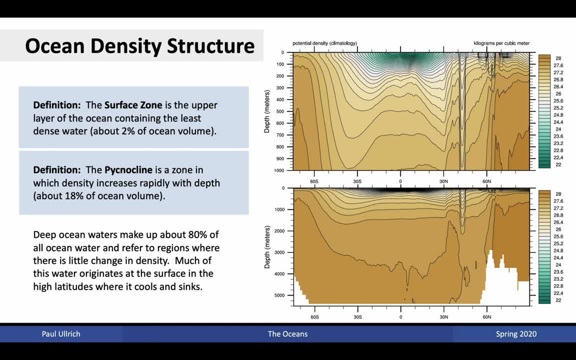 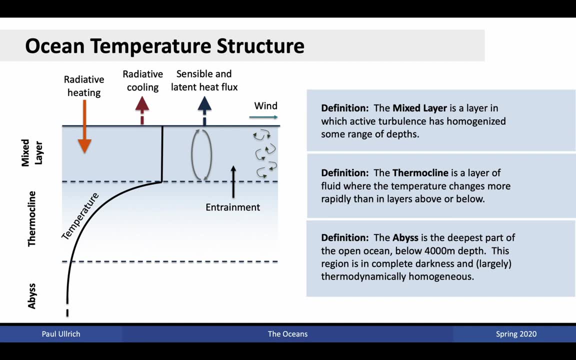 Consequently, that ocean water rarely but is able to produce, essentially, an oceanic convection event leading to an exchange of surface and water at depth. Here's another depiction of the oceanic temperature structure, depicting some of the key processes that are relevant in order to understand ocean dynamics. 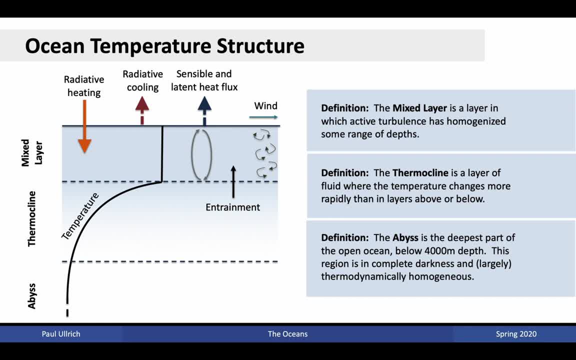 We have radiative heating, which again primarily plays a role near the ocean surface. We have radiative cooling, which is responsible for cooling the ocean surface through terrestrial radiation emission. We have sensible and latent heat flux, so the ocean can release energy to the air through mixing. 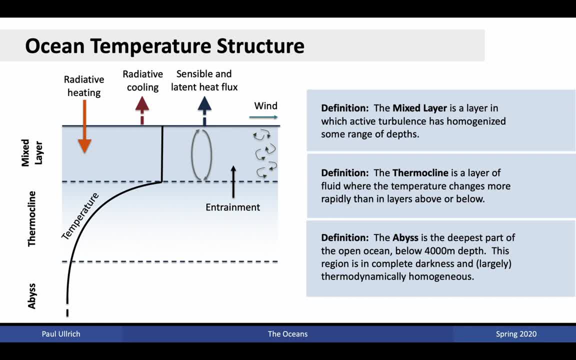 and through conduction to the air, And it can also evaporate, and that evaporation then leads to an overall cooling of the ocean surface, as the more energetic water molecules leave the ocean surface. The wind drives along the ocean surface from the atmosphere. 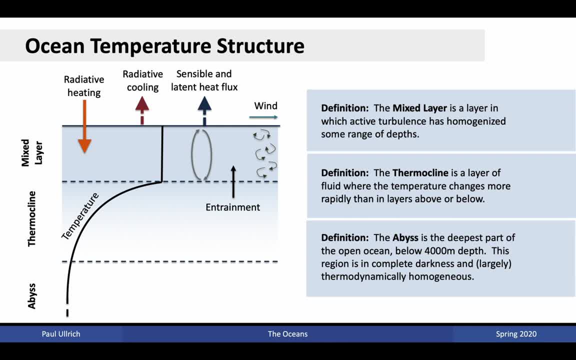 Much of the wind is of course driven by variations in pressure that are in turn driven by variations in temperature due to solar heating. So the atmospheric dynamics then play a role in affecting the ocean surface dynamics through frictional effects. These frictional effects then result in the development 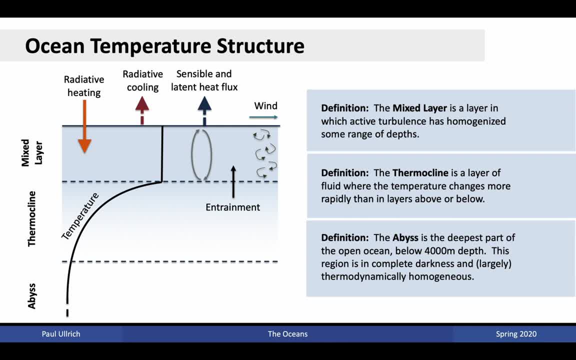 of what is known as the mixed layer of the ocean, which is the top level, which is highly turbulent and homogenized by the presence of this turbulence. Formally, the mixed layer is the layer in which active turbulence has homogenized some range of depths within the ocean. 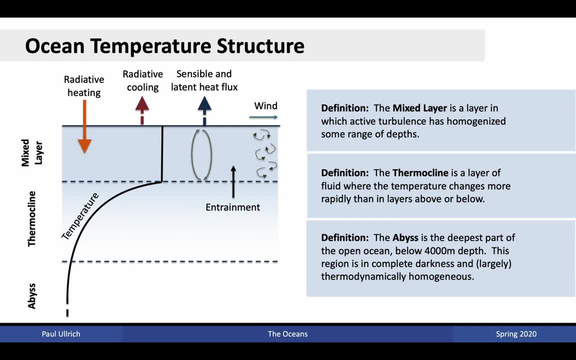 Below the mixed layer we have the thermocline. Much like the pycnocline, the thermocline. this is associated with a change in a thermodynamic quantity. For the pycnocline that change was in density and for the thermocline that change is in temperature. 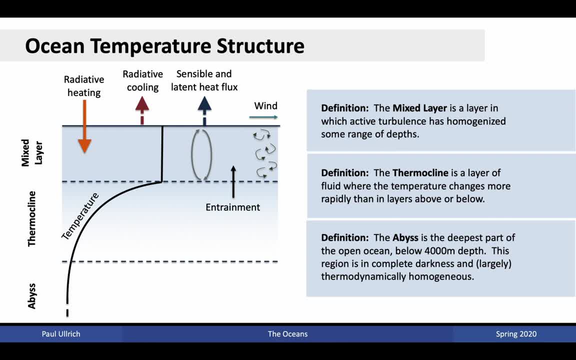 So through this region of the ocean we have a strong drop in temperature as one goes to depth. Finally, in the abyssal region, or the abyss, this is the deepest part of the open ocean, below 4,000 km depth, and it's a region of complete darkness and is largely thermodynamically homogenous. 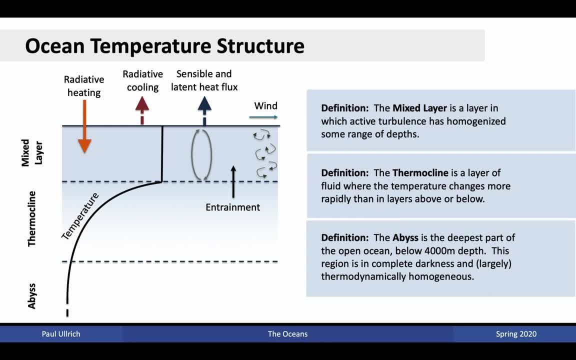 Entrainment at the bottom of the mixed layer is still capable of bringing in water from the thermocline layer and that's important for mixing up, basically, the top of the thermocline with the mixed layer and keeping the two consistent with one another. 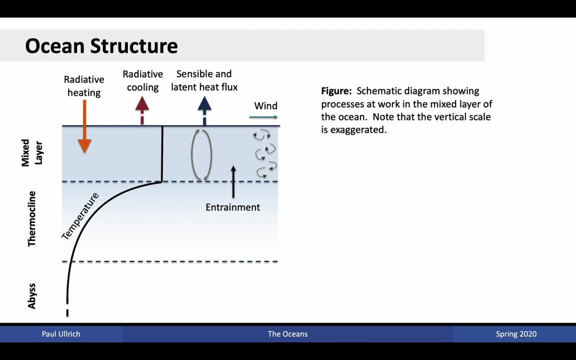 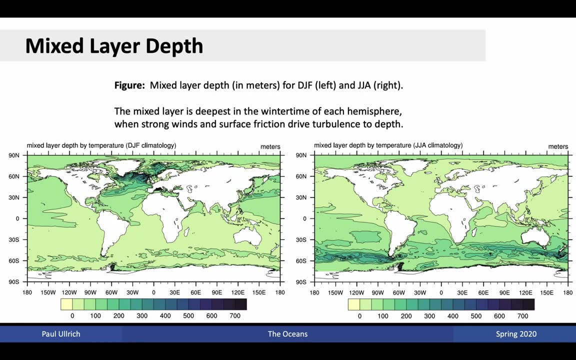 Alright, so note these key processes. As we delve more into our understanding of ocean dynamics, we're also going to work to understand how each of these processes can play a role in driving the ocean dynamics. The mixed layer depth is variable depending on geography. 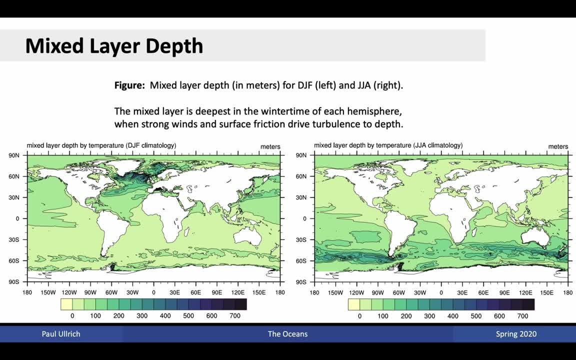 depending on where you are and depending on seasonality, Since the mixed layer is primarily driven by surface friction, where you have the strongest atmospheric winds is also where you tend to have the deepest layers of turbulence, Because the polar jet is primarily responsible for driving the strongest near-surface wind speeds over the ocean. 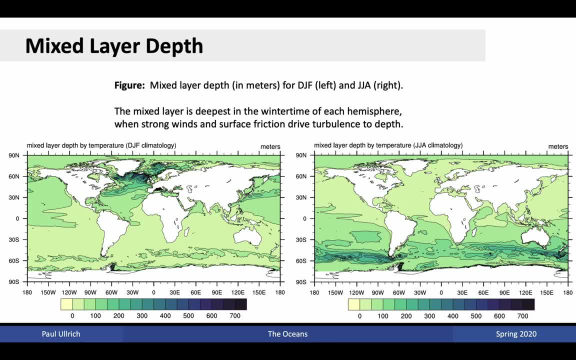 we also find that that polar jet region also tends to be where the mixed layer depth is the deepest, In particular on the left-hand side. here we have the Northern Hemisphere wintertime climatology of the mixed layer depth and what we see is that 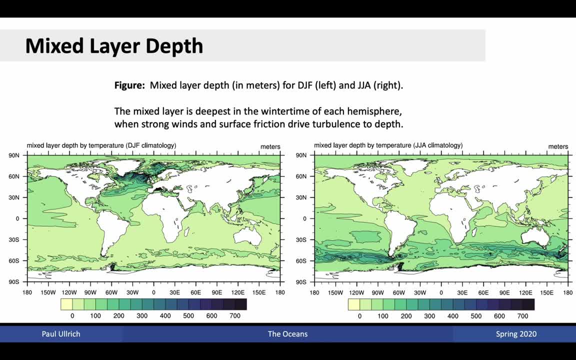 the mixed layer depth can drop to 500 or 600 meters climatologically in some of the regions that have the strongest atmospheric winds. So we have the strongest atmospheric wind speeds driving turbulence in the near surface. In the Southern Hemisphere again, we see a very pronounced 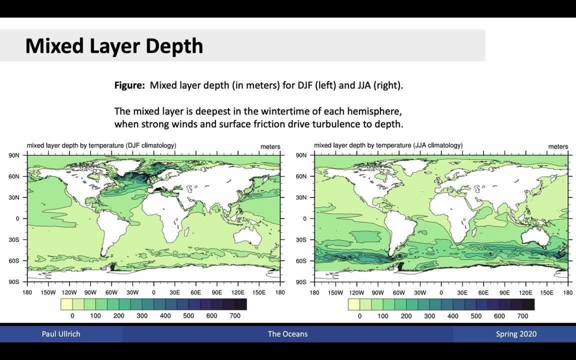 mixed layer depth that occurs during the Northern Hemisphere summertime, Southern Hemisphere wintertime. This primarily occurs along the Antarctic Circumpolar Jet, and this is responsible for then producing in the oceans what is known as the Antarctic Circumpolar Current, which is a region of very strong westerly motion. 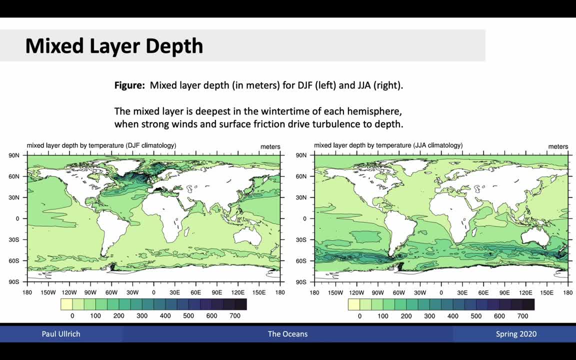 in the ocean and is highly turbulent, particularly over the Southern Hemisphere winter season, driving very deep mixed layer depths. The overall magnitude of this mixed layer depth is important for understanding mixing within the ocean and so just understanding that typical values of this around 100 to 200 meters outside of these heavily mixed regions. 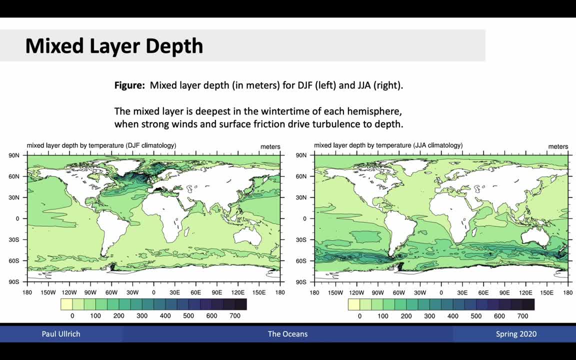 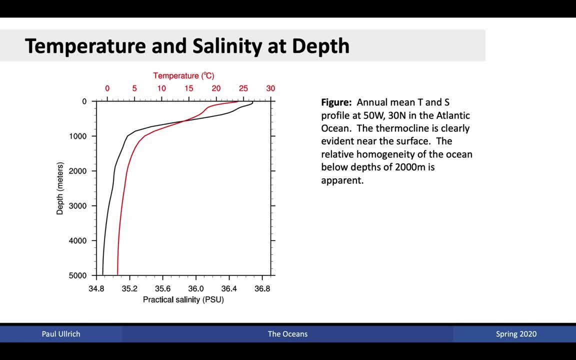 and 500 to 700 meters in kind of the more heavily mixed regions is important. Looking at vertical structure at a few points within the ocean, here we see the vertical temperature and salinity structure: Temperature shown in red, salinity shown in black. 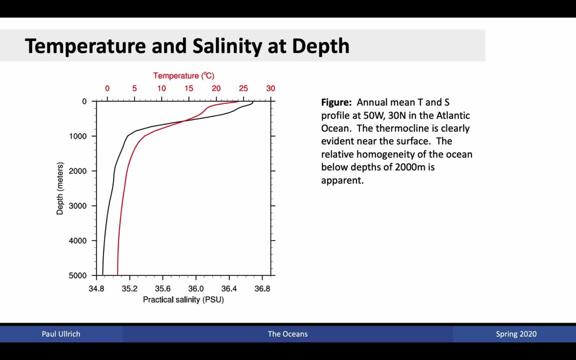 As you can see, near the top of the ocean we have very rapid variation in both of these parameters. In particular, temperature varies very close to the near surface in that top 200 meters or so, whereas salinity appears to be a little bit more well mixed with depth, until you get basically. 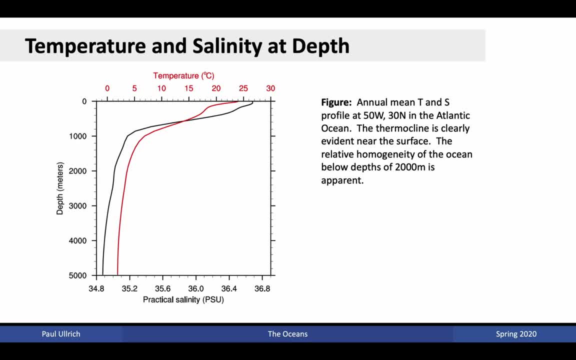 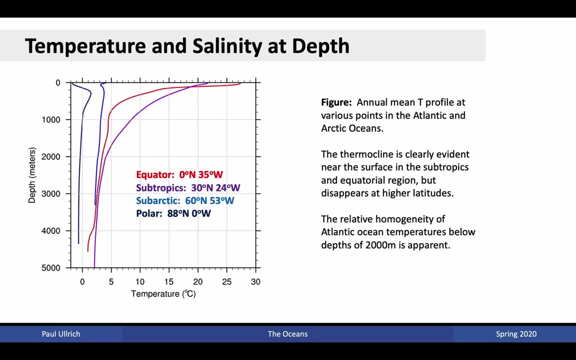 to this thermocline region below 200 meters where you have a rapid drop off in temperature before reaching at about 2000 meters, basically a fairly homogenous region for both temperature and salinity. Here are profiles of temperature at various points throughout the Atlantic and Arctic oceans. 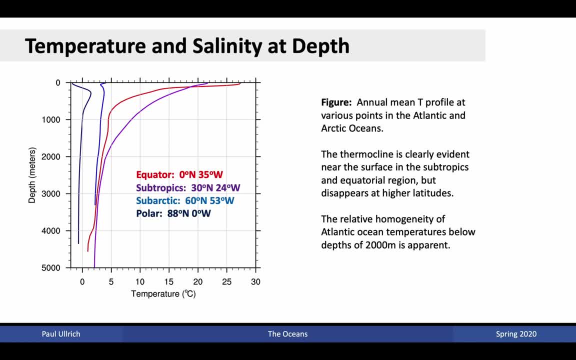 In red we see the equator. In purple we see the subtropics. In blue the subarctic And in dark blue the polar regions, taken essentially near the ocean. This is near the North Pole. What we see here is in the equatorial regions. 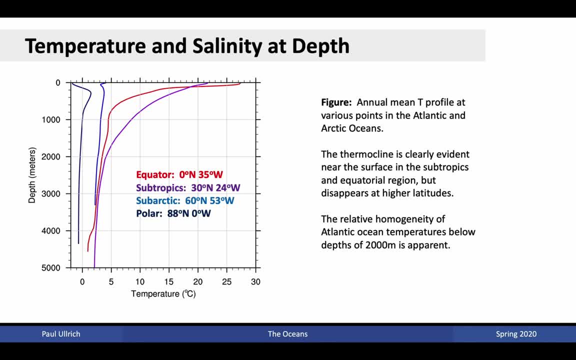 we have the highest temperatures, but we also see a very rapid drop off in those temperatures as we go to depth. This is because there's not a lot of pumping to depth, That is, you don't have a lot of mixing of near surface waters. 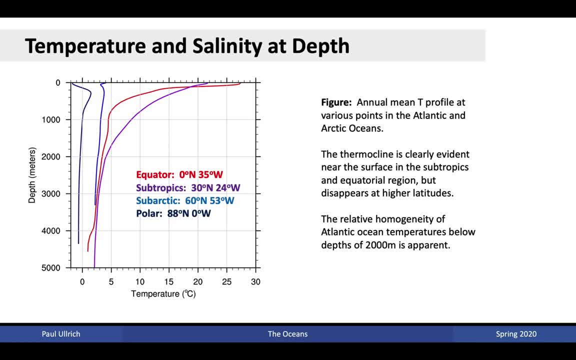 and ocean waters at depth, and so those ocean waters a little bit under the equatorial surface tend to be not in contact and not be influenced by near surface radiative forcing. On the other hand, in the subtropics, at 30 degrees north, 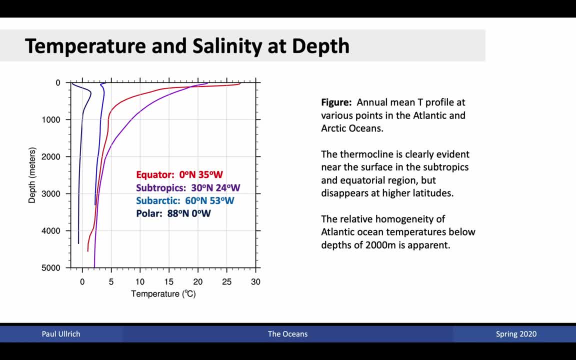 we do have pumping to depth. So, even though the surface temperatures are cooler, as one would expect in accordance with radiative forcing, at the near surface we do have warmer temperatures at depth, as those near surface waters are pushed downward, And so we'll understand that in a couple lectures' time. 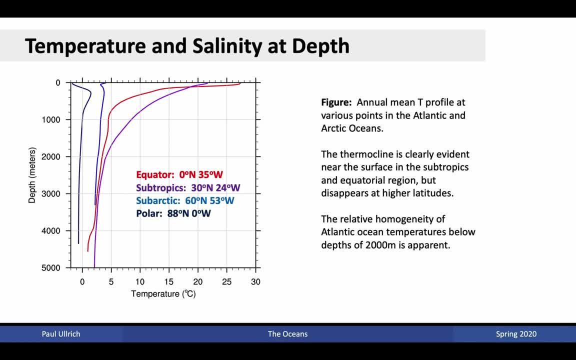 In the northernmost latitudes, that is, in the subarctic and polar, we actually don't have much of a thermocline at all. In fact, the temperature profiles appear to be very similar with depth. Part of this is because there is more significant mixing. 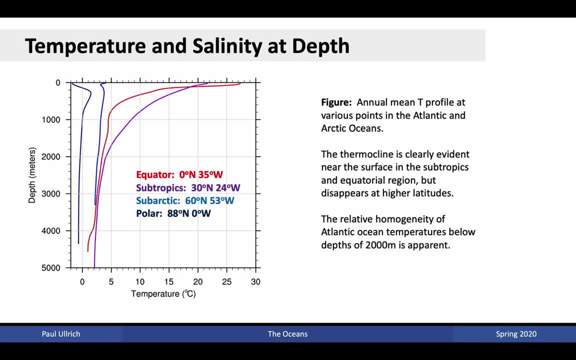 that is occurring at these depths, That is, with a constant temperature profile, we tend to have stratification that is closer to neutral stratification, which has the potential to induce then convection within the oceans and push those surface waters to depth. 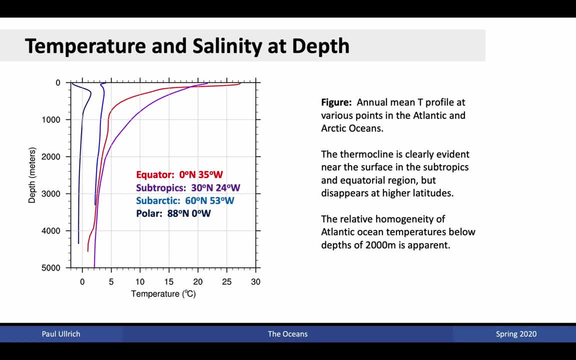 where we get more homogenization then of the temperature profile. Part of it is also the removal of heat from the near surface, as we see in the polar plot here, where the deeper layers of the ocean are actually maintained at warmer temperatures because the polar region 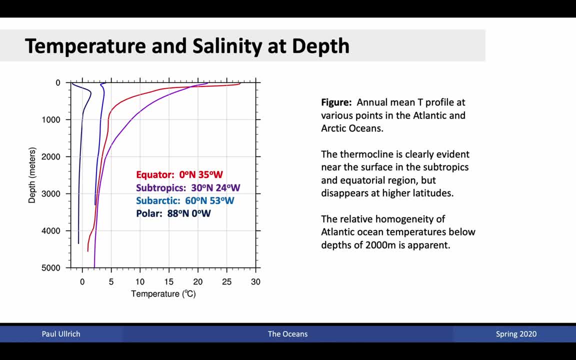 is basically losing all of its heat to the atmosphere and to radiative outputs. However, once one gets below about 2,000 km depth, the overall structure of the ocean is fairly homogenous, All of the three lines that emerge from the Atlantic. 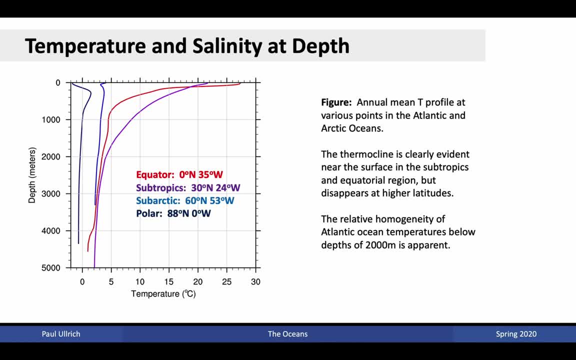 all seem to have essentially the same profile, regardless of where they are. There are some differences at the bottom, but that varies primarily because of the differences in bottom topography. The polar region is also homogenous, but is at a cooler temperature. 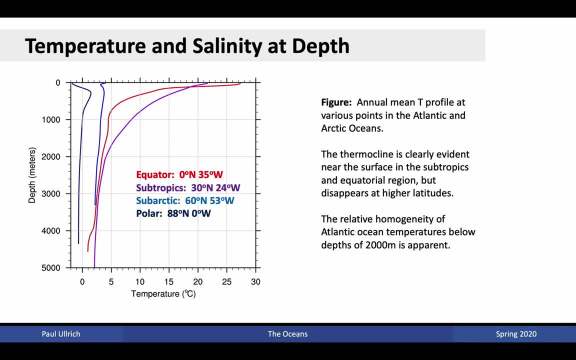 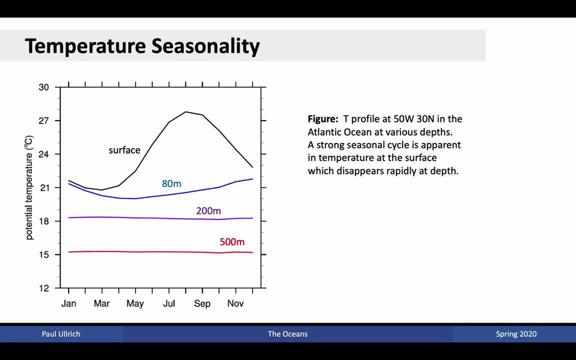 because the Arctic is a little bit more isolated than these three lines taken from the Atlantic. The seasonality of ocean temperatures is not particularly severe. compared to the changes in seasonality that one saw in the atmosphere At the near surface, we do see more change in temperature. 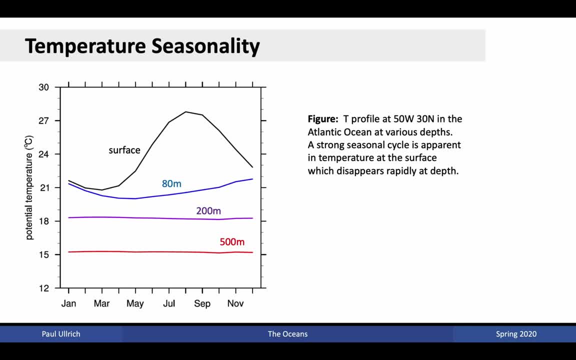 as one might expect for a region that is directly exposed to radiation. but even getting to 80 m depth, which is still within the mixed layer, one sees much more homogenous temperatures regardless of season, And in fact we see a shift in that seasonality. 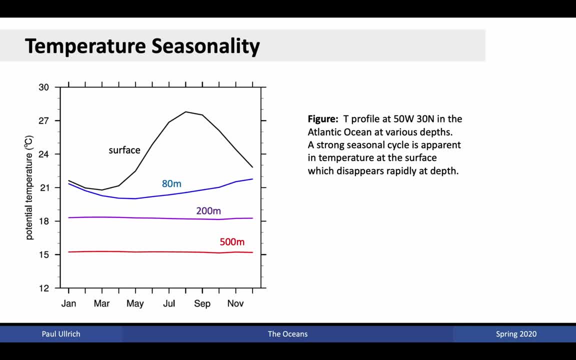 where you have warmer temperatures actually occurring closer to November and December than you do at peak radiative temperatures in the summer time. Below 80 m depth, we see temperature profiles that are effectively constant, and this is again because there is no real mechanism by which these surface ocean waters. 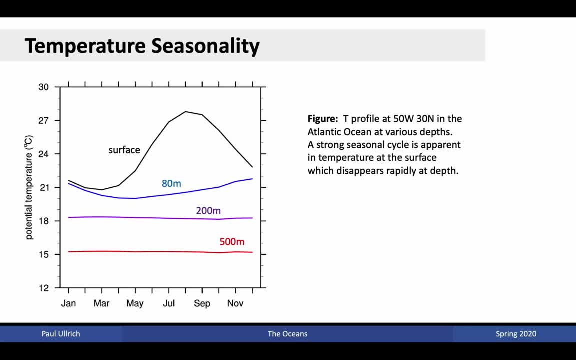 can communicate with ocean waters at depth except through deep convection, which doesn't really occur in the equatorial regions. So these waters tend to remain isolated and remain at fairly constant temperatures throughout time. By the time you reach 200 m depth, 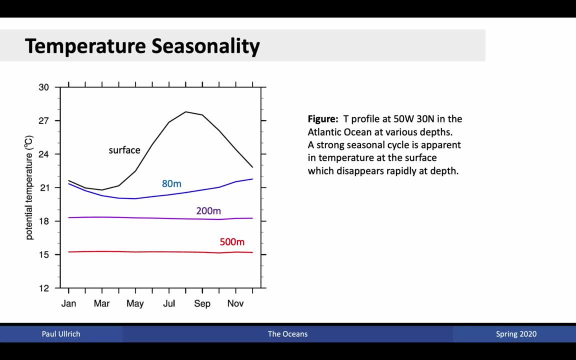 you basically have removed almost all of the incoming radiative forcing, the incoming solar forcing, so that solar forcing has very little effect at changing the ocean temperatures. Further the thermal effects of ocean water, that is, the fact that it tends to be resistant. 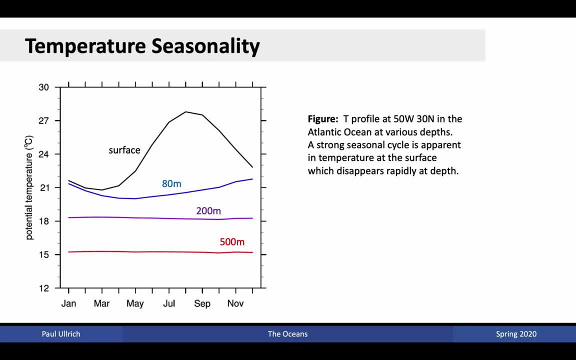 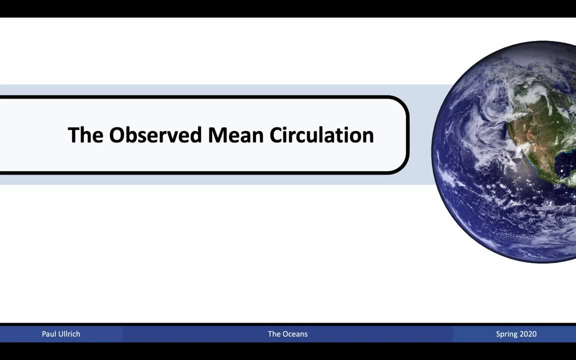 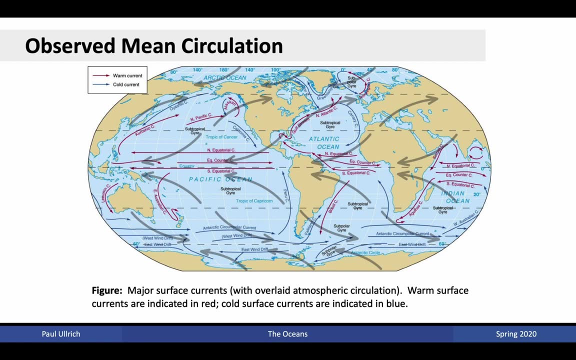 to temperature change plays a role in affecting this temperature seasonality. Alright, let's talk about the observed mean circulation, that is, how exactly ocean currents are moving around the globe. Here's a depiction of the observed mean circulation of ocean currents, shown with the primary branches: 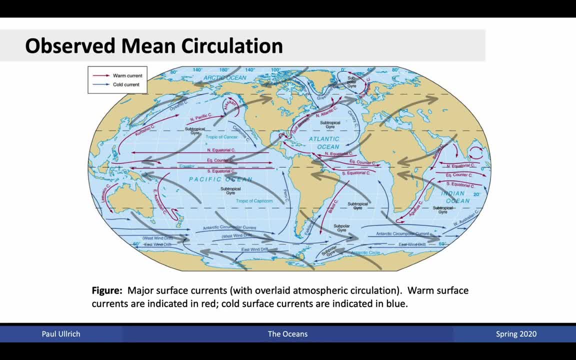 of the large-scale circulation superimposed in the grayish arrows. The red arrows here depict warm ocean currents- that is, where warmer waters are circulated into cold regions, and the blue lines- blue arrows- show cold ocean currents. that is where colder, poleward ocean water. 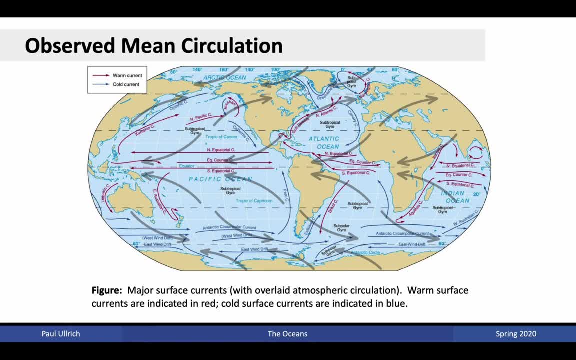 is being pushed into the equatorial regions. There are a couple interesting results from this figure. In particular, notice the presence of the easterly equatorial current and both the northern equatorial current and the southern equatorial current. that seems to be present in each of the. 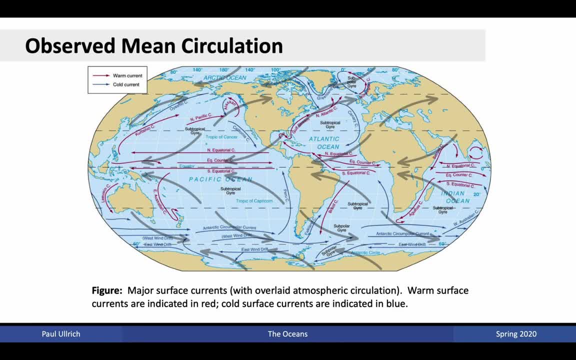 three major ocean basins. We see it in the Pacific, the Atlantic and the Indian. However, unlike the atmosphere, there's also an equatorial countercurrent, which is this arrow shown going from left to right. This is actually a westerly. 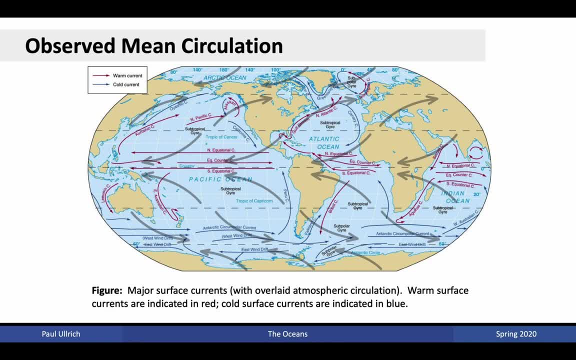 that is, it comes from the west, that propagates in between the north equatorial and south equatorial current, And this is a really interesting feature of the oceans that we'll get into in a little bit more detail in three lectures' time. 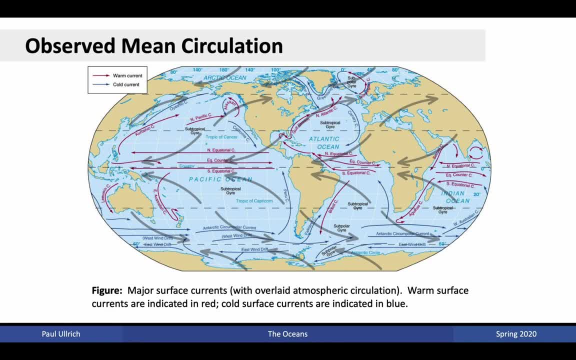 Overall, the oceanic circulations are not unlike the atmospheric circulations. We see again easterlies closer to the equator and westerlies farther north. So it is perhaps not unexpected that these oceanic circulations follow in accordance with what we would expect. 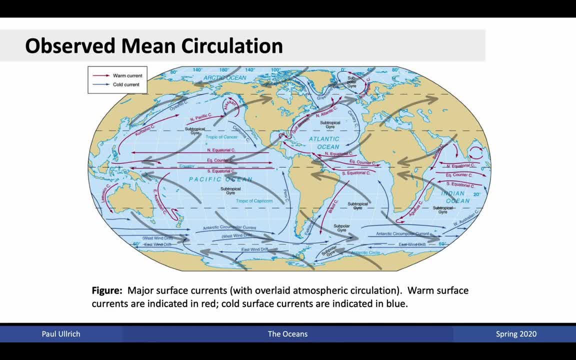 for geostrophic flow. The large circulations here are known as the subtropical gyres, and they're responsible for driving warmer waters poleward along the western edges of these oceanic basins and colder waters southwards along the eastern edges of the basins. 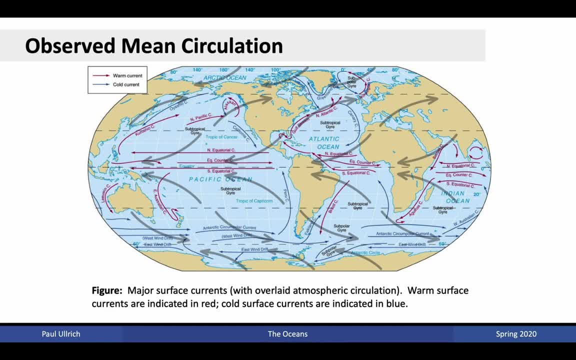 Unlike the atmosphere, again, we have laterally bounded conditions which are at the edge of each basin, which means that these circulations need to be self-contained within every basin, So you're not going to be able to blow over land and consequently you need to. basically, 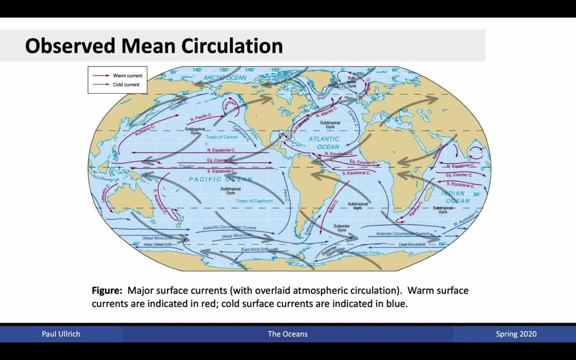 circulate the ocean waters. The primary driver for these circulations is the wind, So you'll notice that there's pretty good agreement between the wind vectors and the underlying currents. This works pretty much everywhere, except for the equatorial countercurrent, which is a weird anomaly, as mentioned. 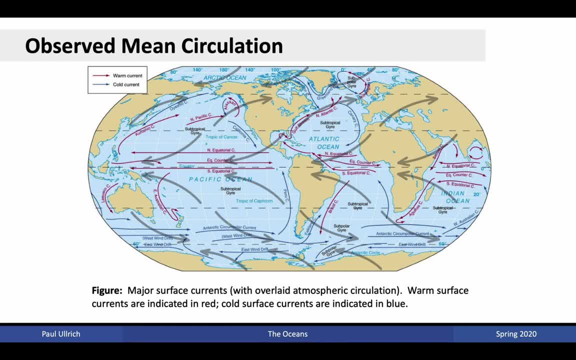 The strongest circumpolar currents occur in the Antarctic, known as the Antarctic circumpolar current, and it is this region of westerlies that are present basically around the Antarctic continent And they continue to circulate fairly rapidly around this region. The overall currents that we see here: 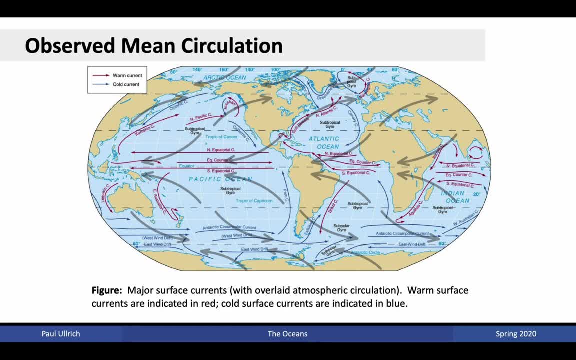 are also responsible for exchanging waters between different ocean basins, although, again, the mechanisms to do so basically require going through them, going through particular regions of the oceans. That is the only way in which the Atlantic, Indian and Pacific can really exchange their waters. 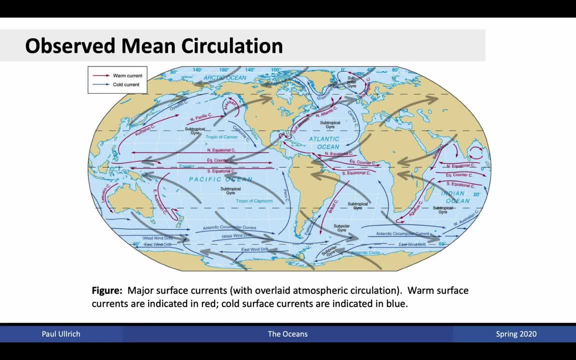 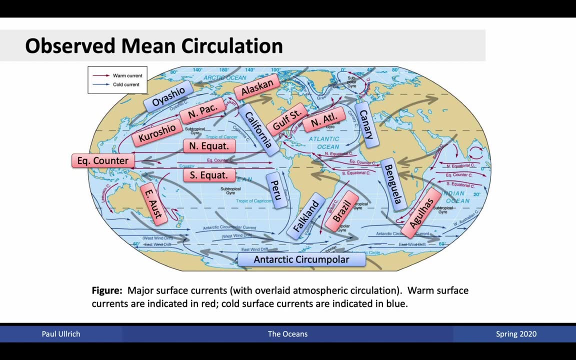 is through this Antarctic circumpolar current. A little bit of leakage does occur through the Bering Strait, which allows Pacific waters to seep into the Atlantic, but this is a much slower process with much lower volume associated with it. Here are the names of these various currents: 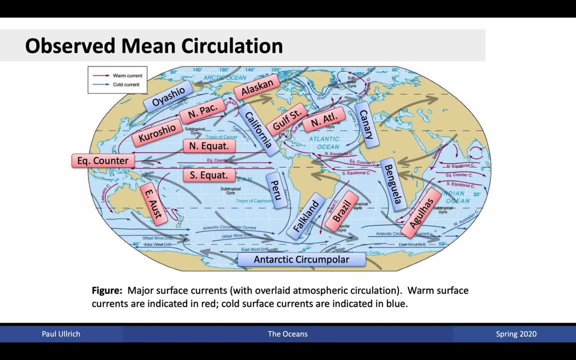 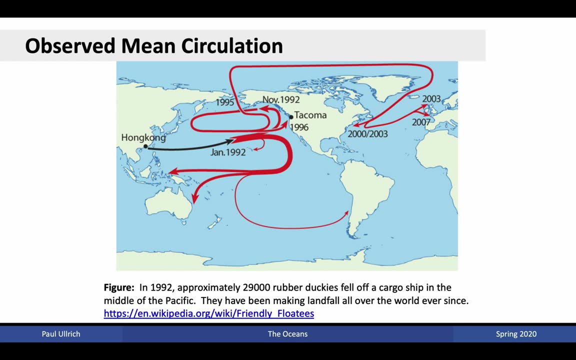 overset on this particular image. I don't necessarily encourage you to memorize all these unless you're into oceanography, but here they are for reference. In order to understand this oceanic circulation, a unique experiment was actually performed in 1992, not intentionally. 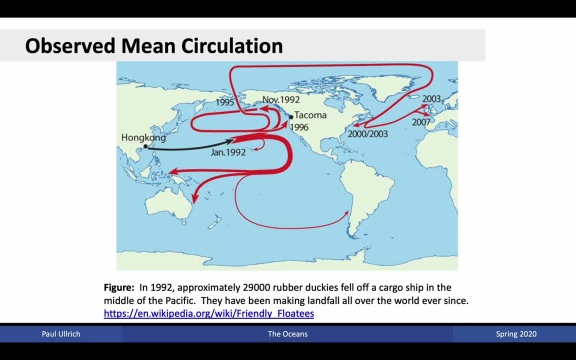 but during this time, a cargo ship that was traveling from Hong Kong towards North America was carrying along with it approximately 29,000 rubber duckies. As the ship was transiting the Pacific, this cargo container of rubber duckies fell off the ship. 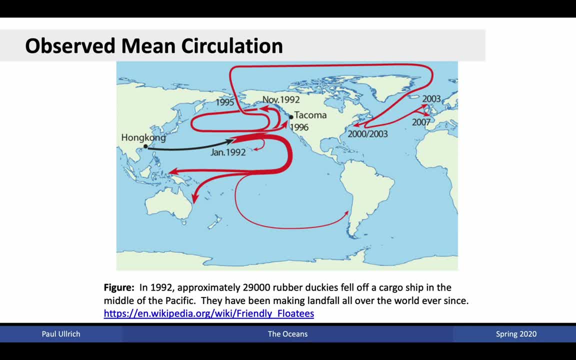 and the rubber duckies were left free to float in the Pacific Ocean. This provided us with a very unique opportunity in order to assess the eventual fate of the rubber duckies and where the ocean eventually blew them. The various locations at which these rubber duckies. 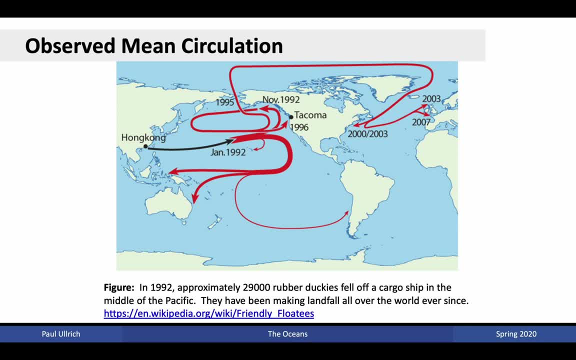 made landfall allowed us to understand how quickly the ocean water circulated. So in the Pacific some of these were seen to make landfall in 1992 in Alaska and 1996 in Washington State, likely a product of circulating around one of these northern Pacific gyres. 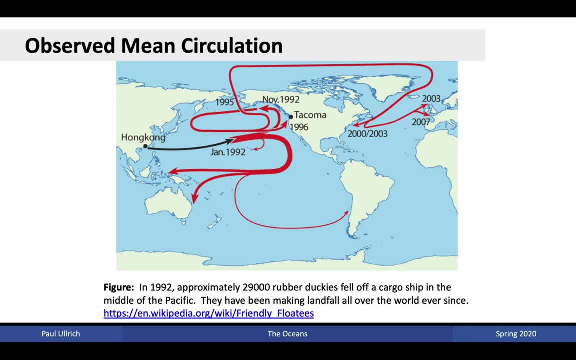 and passing through the Bering Strait in 1995, before transiting and finding themselves in Europe and along the eastern coast of North America in the 2000s. We also saw these rubber duckies wash up on shore in equatorial regions along the maritime continent. 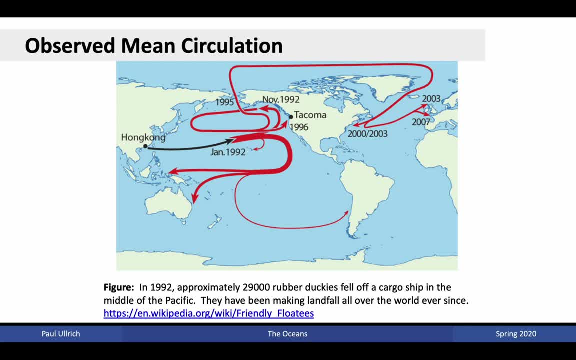 as well as a couple that even passed into the southern hemisphere and washed up in South America. This was a very valuable opportunity in order to understand these oceanic circulations, and I encourage you to read more about this on the Wikipedia page on Friendly Floaties. 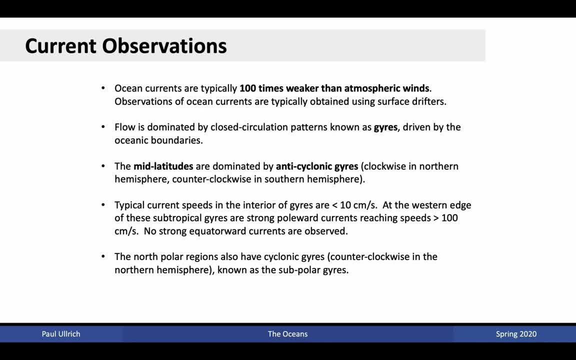 Alright, so what did we observe about the currents in the previous two plots? Ocean currents, we know, are typically about 100 times weaker than atmospheric winds, That is, they move very slowly compared to corresponding atmospheric wind speeds. Observations of these ocean currents. 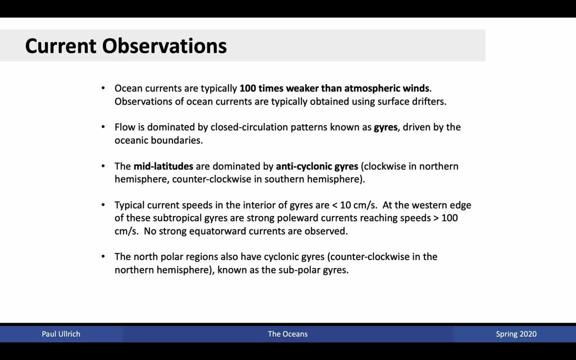 are typically obtained using surface drifters. so by putting a GPS system onto a floatie and setting that out into the ocean, we can track its position and understand how rapidly the objects are being pushed around along the oceanic surface. The large-scale circulation in the ocean. 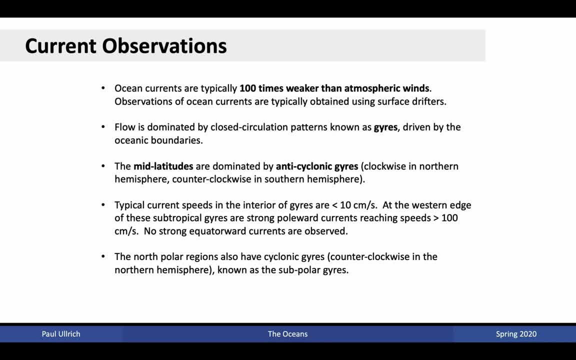 is dominated by closed circulation patterns, known as the oceanic gyres, which are driven by oceanic boundaries but are also driven by the wind-driven circulation, That is, wind friction is responsible for driving these currents at the surface and they agree consequently. 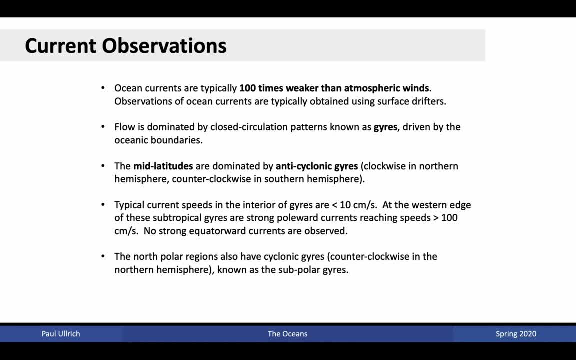 pretty well with the atmospheric circulation. The mid-latitudes are dominated by anti-cyclonic gyres, so these tend to move clockwise in the northern hemisphere and counterclockwise in the southern hemisphere- Typical current speed in the interior of these gyres. 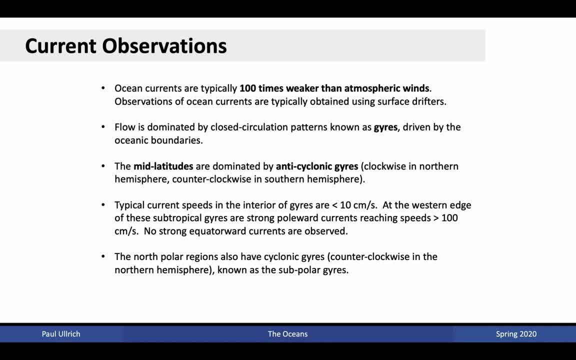 is less than about 10 cm per second, but close to that level, At the western edge of these subtropical gyres, we have what are known as strong western boundary currents, which tend to reach speeds in excess of 100 cm per second. 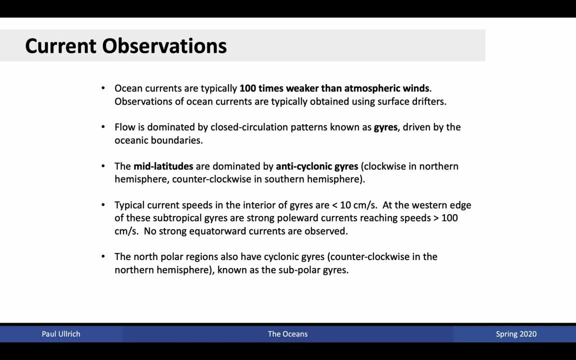 These western boundary currents do not have corresponding eastern boundary currents that are responsible for transporting flow from a pole to an equator, so they're fairly unique. We'll understand why that's the case in a couple lectures' time. These western boundary currents 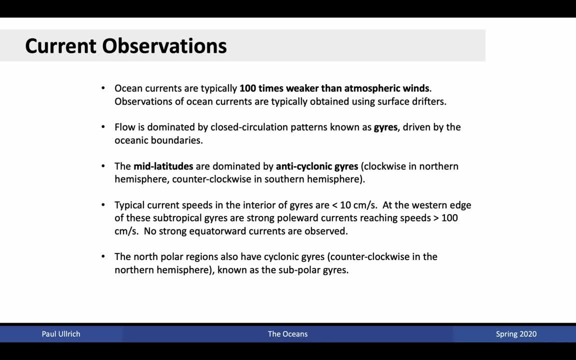 which include the Gulf Stream, are then responsible for pushing quite a bit of heat from the subtropics northward through the oceans, and thus are a major contributor to this poleward heat transport of the climate system. The north polar regions also have cyclonic gyres. 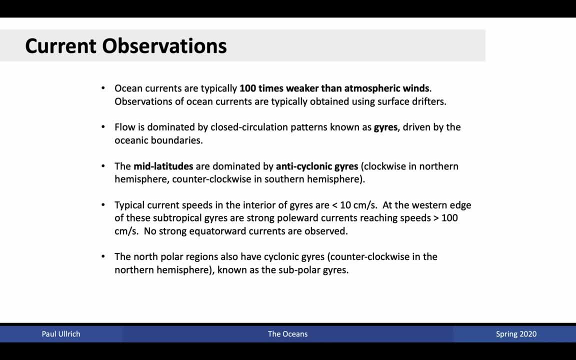 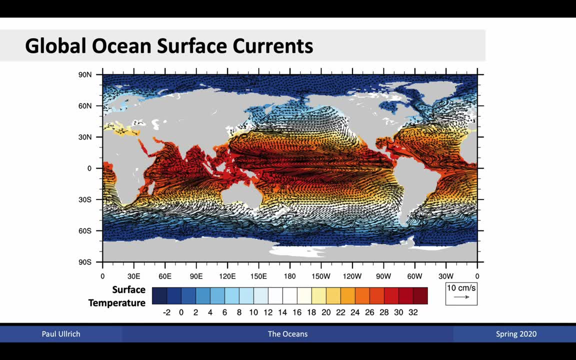 that is counterclockwise in the northern hemisphere, which are known as the subpolar gyres, but you have to get to pretty high levels of latitudes in order to see these. Here's another image showing global surface currents using tracking vectors. 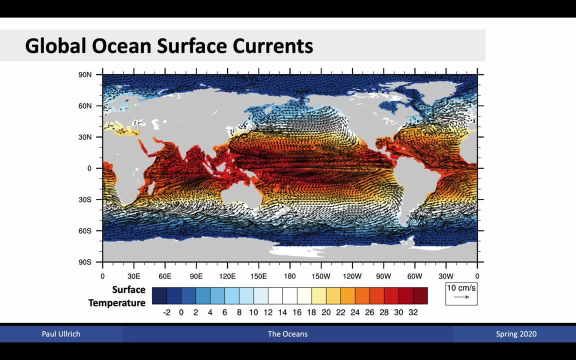 and with temperatures overlaid. A few things worth keeping in mind here. First of all, we see the presence of the equatorial and equatorial countercurrents. We see the strong western boundary currents that emerge in this diagram where we see these vector lines. 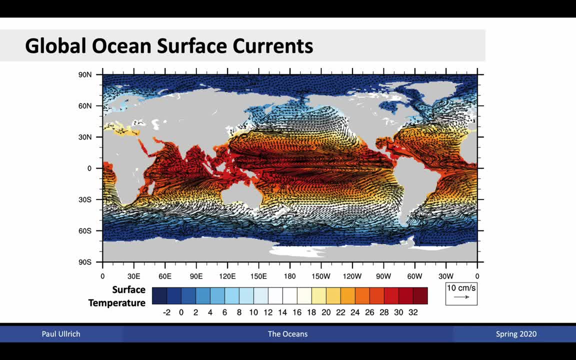 laying very tight with one another. Similarly strong western boundary currents in the southern hemisphere, along the coast of South America and along the coast of Africa. We also see a really strong Antarctic circumpolar current. Let's look at these in a little bit more detail. 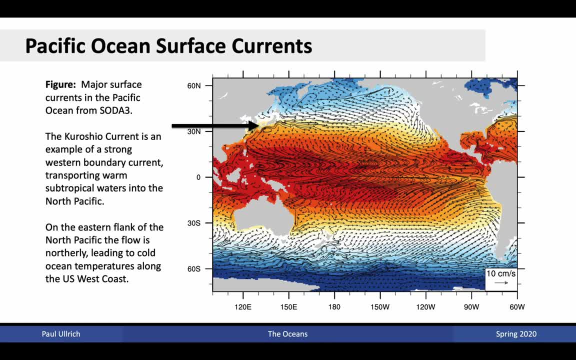 Here we see the Pacific Ocean In particular. the Kuroshio Current is an example of one strong oceanic western boundary current, and that one comes along the coast of Japan before exiting into the North Pacific. Again, this is the western branch. 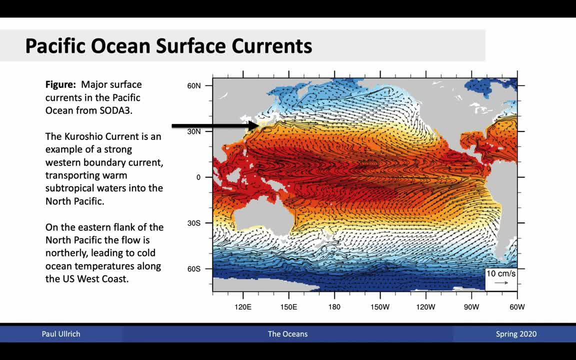 of the northern Pacific subtropical gyre. This is responsible for transporting these warm subtropical waters into the North Pacific. Along the eastern branch of the Pacific, however, you see no such pattern, no such strong circulation. However, the flow is nonetheless northerly. 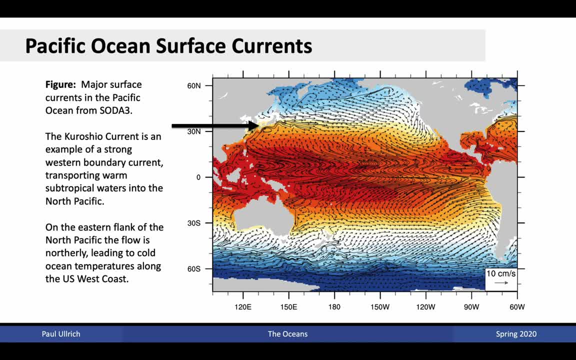 pushing colder ocean waters further south. This is then responsible for cooler temperatures that are experienced along the western coast of North America as compared to corresponding latitudes in Asia. The equatorial countercurrent shows up prominently in this diagram, which is a western current. 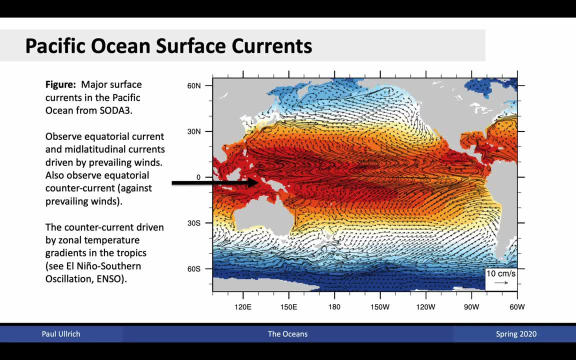 basically passing almost directly at the equator. It's driven by zonal temperature gradients in the tropics and is closely connected also with the El Niño Southern Oscillation. The equatorial currents are associated with prevailing winds, that is, since we primarily have 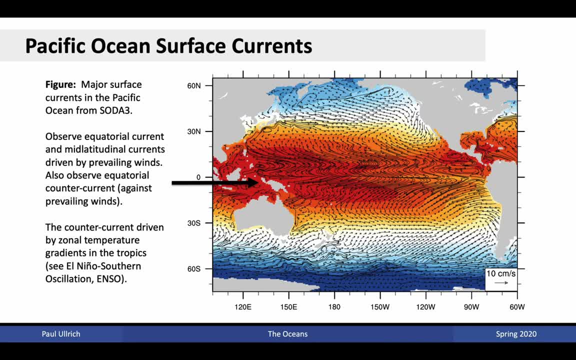 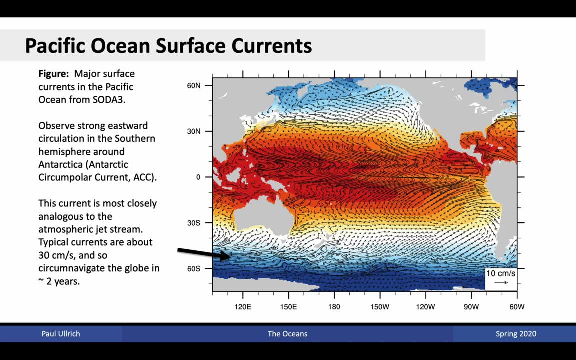 easterly winds associated with the returning branch of the Hadley Circulation. these then drive easterly circulations in the oceans And finally, as mentioned previously, the Antarctic Circumpolar Current, or the ACC, pops up quite prominently in this figure. 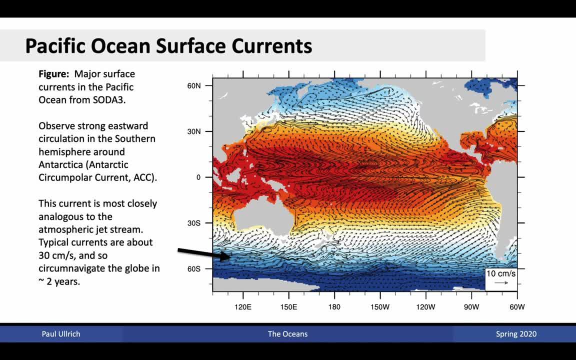 as it passes around Antarctica. The current is probably the most close analog in the ocean to the atmospheric jet stream, with typical current values reaching about 30 centimeters per second. So for a particular fluid parcel to circumnavigate the Gold River or circumnavigate the globe around the ACC, 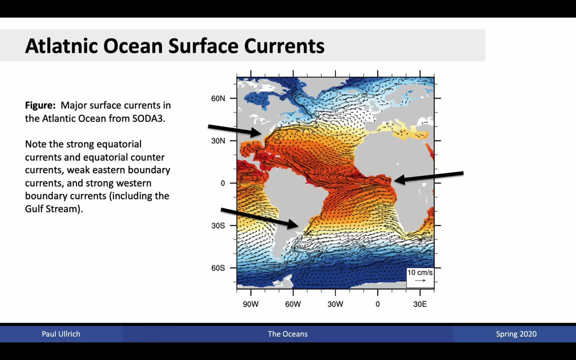 it takes about two years. Here's a look in the Atlantic Again, we see a strong western boundary current known as the Gulf Stream. We also see in the Labrador Sea, towards the top of the diagram, the Labrador Current which is responsible for pumping. 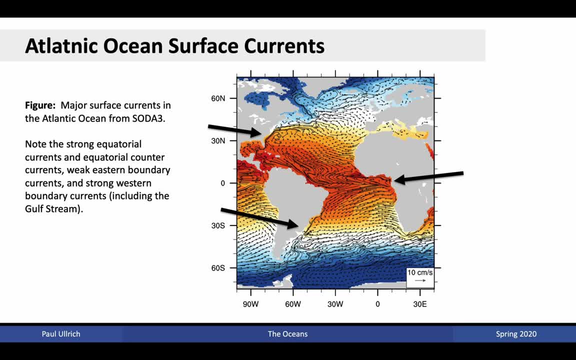 colder ocean waters into the North Atlantic. Note also that we have a strong western boundary current along the east coast of South America, here known as the Brazil Current, And we also see again the presence of both the north equatorial, south equatorial. 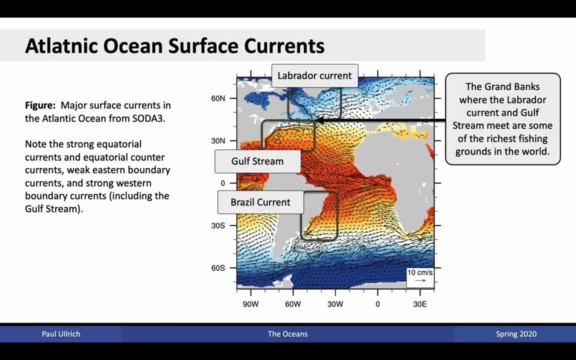 and equatorial counter currents. in this diagram, As mentioned, we see the Gulf Stream, Brazil Current and Labrador Current. In this region, where the Labrador Current and the Gulf Stream connect with one another is known as the Grand Banks off the coast of Canada. 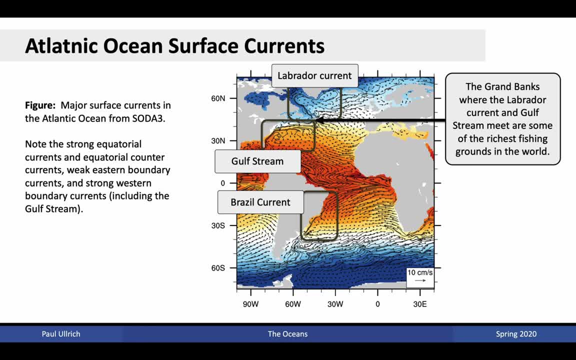 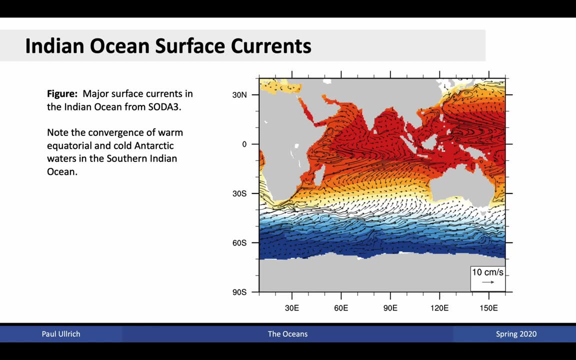 And this is also one of the richest fishing grounds in the world because of sediment transfer that makes this region particularly rich in sea life. Finally, looking at the Indian Ocean again, we see the Antarctic Circumpolar Current, we see the equatorial currents. 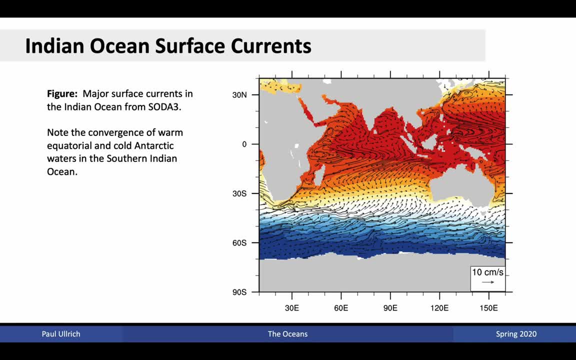 and the equatorial counter current. Much of the circulation here is inputs from the warm Pacific waters and over the maritime continent and we see a slow flow of surface waters southward at this point and a convergence of warm and cold waters occurring basically along the western coast. 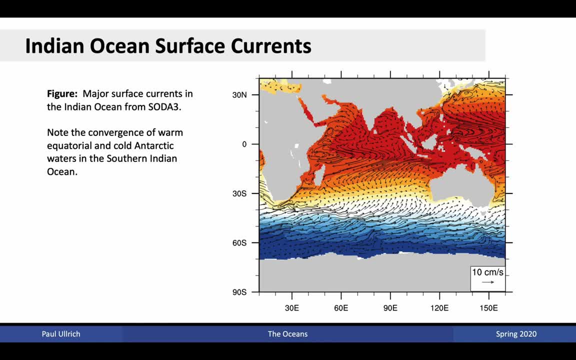 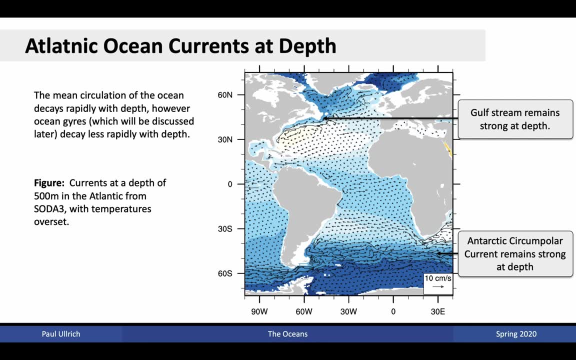 of Australia stretching to the southern tip of Africa. If we look at these currents at depth- here is a depiction at 500 meters depth in the Atlantic- We see that the speeds of the currents have dropped off dramatically, and this is a well-known feature within the ocean.